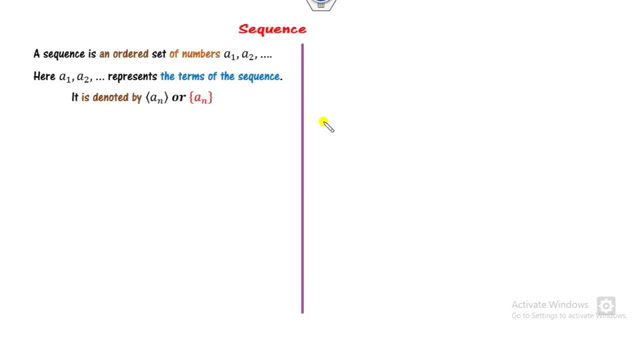 mathematics. What is the sequence? As we discussed in our last lecture, sequence is the set of the ordered numbers, which is denoted by a1, a2 and so on, and the sequence is denoted by curly braces of a1 or r, like here: If this series is my finite, then we call as the finite sequence. If it is. 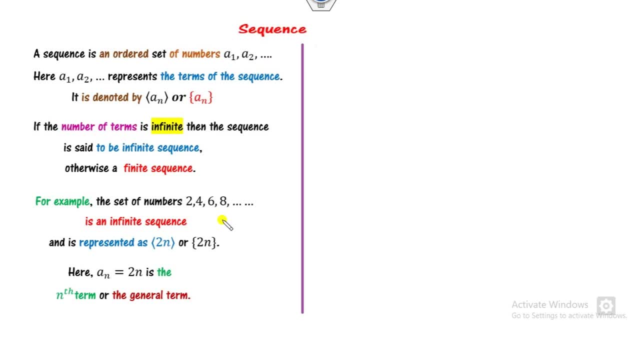 infinite, then we call as the infinite series. For example, if you consider the set of the even numbers 2,, 4,, 6 and 8, and this the nth term of this sequence is denoted by a1 and this is the sequence of it Now, since they are the infinite terms, so we can call as the infinite sequence. 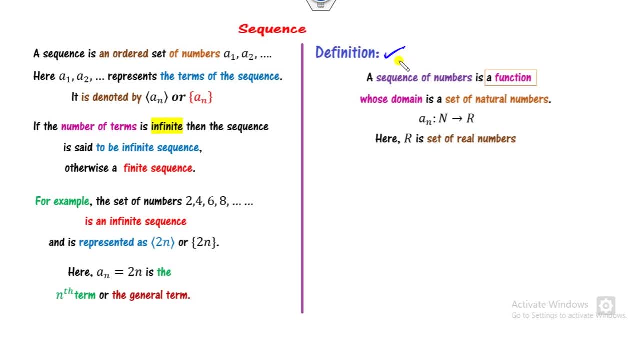 Based on this, we can define the formal definition of the sequence. A sequence is a function whose domain is a sequence. A sequence is a function whose domain is a sequence. A sequence is a set of the natural numbers, So remember that n is my natural numbers, like 1,, 2,, 3 and so on. This 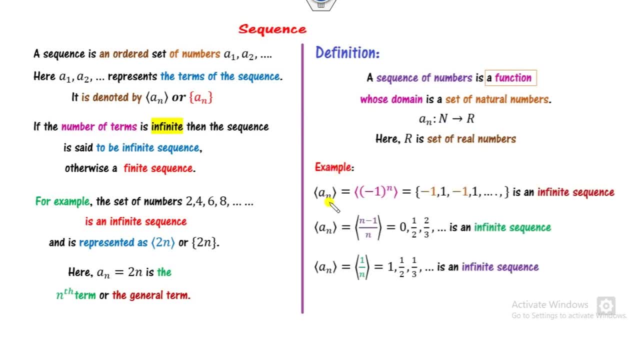 is the most important thing. Based on this sequence, we can define like: of minus 1 raised power n, and so on. Now again, you can see this is an infinite sequence. we call as here. Now, our target of this lecture is to check whether this sequence of this, this or this are monotonic, increasing or 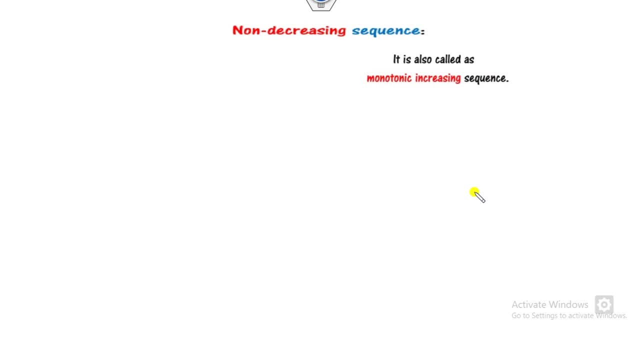 decreasing. So for that we will firstly define the term called as non-decreasing sequence. It is also called as the monotonic increasing. So what is the meaning of the increasing? It means, if I take the first sequence number as a 1, another number as a 3,. 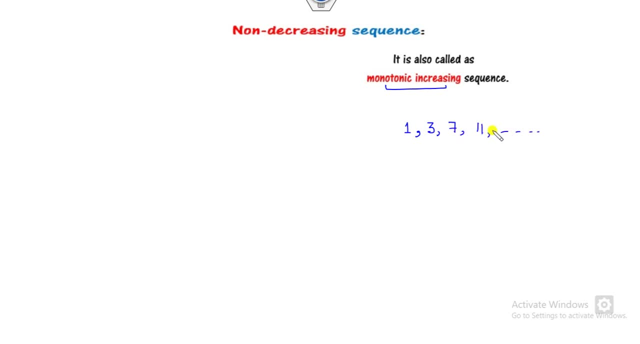 another number. next number is 7, then 11, and then so on, or say 13 then 14.. You can see these are my increasing sequence. The same definition we can apply here: A sequence, an, is said to be the non-decreasing or increasing whenever the next term is greater than of the previous one or you. 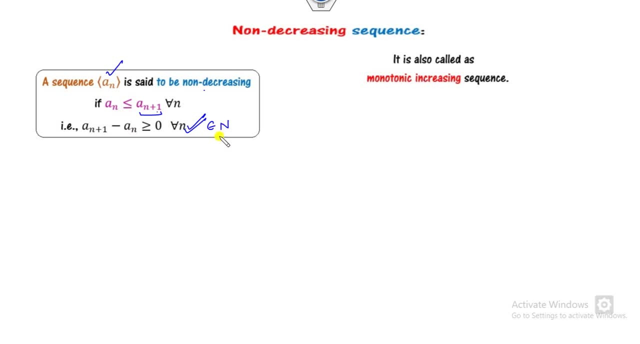 can say n is greater than 0 for all n in the domain natural number. Another definition is: we can say a sequence: an is said to be the non-decreasing if the ratio of the next term to the previous term is always greater than 1 for all n in the natural number. Similarly, if you look about this sequence, 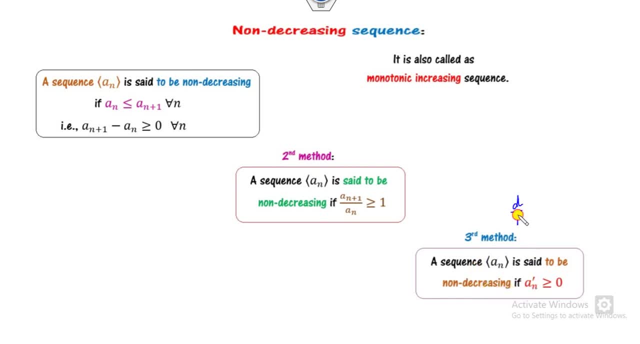 is said to be the non-increasing if the derivative of this sequence with respect to n is my greater than 0. Then we can say it is a increasing sequence. For example, if I try to check whether it is a non-decreasing or not, we will apply that all. 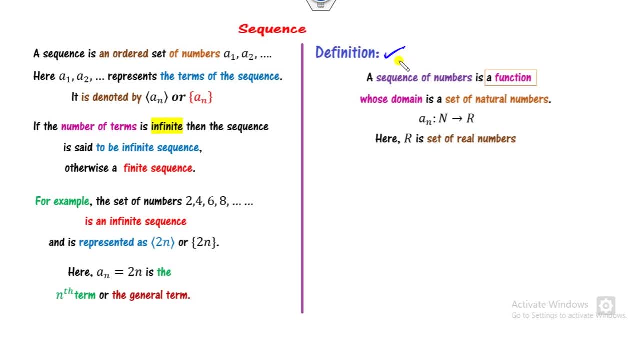 Based on this, we can define the formal definition of the sequence. A sequence is a function whose domain is a sequence. A sequence is a function whose domain is a sequence. A sequence is a set of the natural numbers, So remember that n is my natural numbers, like 1,, 2,, 3 and so on. This 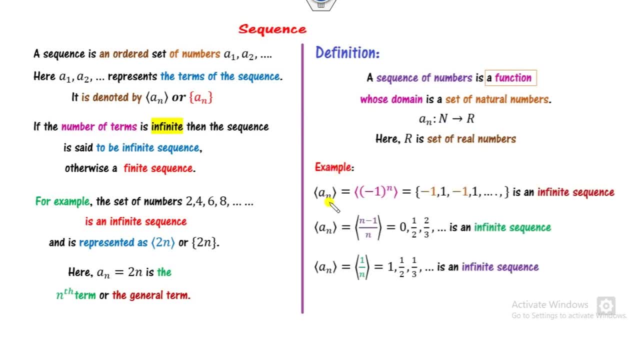 is the most important thing. Based on this sequence, we can define like: of minus 1 raised power n, and so on. Now again, you can see this is an infinite sequence. we call as here. Now, our target of this lecture is to check whether this sequence of this, this or this are monotonic, increasing or 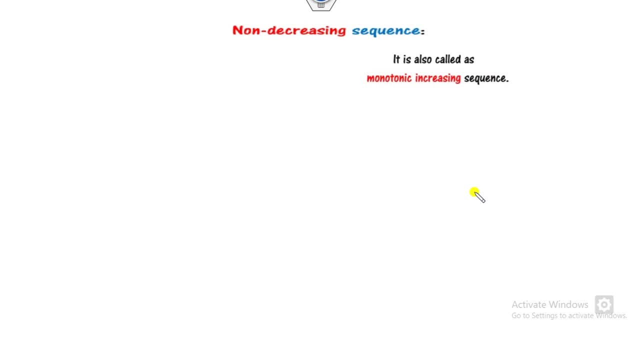 decreasing. So for that we will firstly define the term called as non-decreasing sequence. It is also called as the monotonic increasing. So what is the meaning of the increasing? It means, if I take the first sequence number as a 1, another number as a 3,. 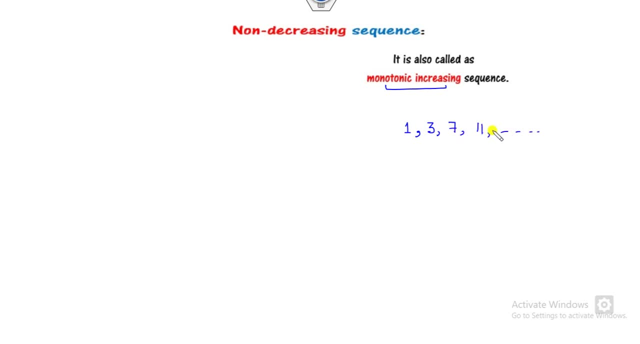 another number. next number is 7, then 11, and then so on, or say 13 then 14.. You can see these are my increasing sequence. The same definition we can apply here: A sequence, an, is said to be the non-decreasing or increasing whenever the next term is greater than of the previous one or you. 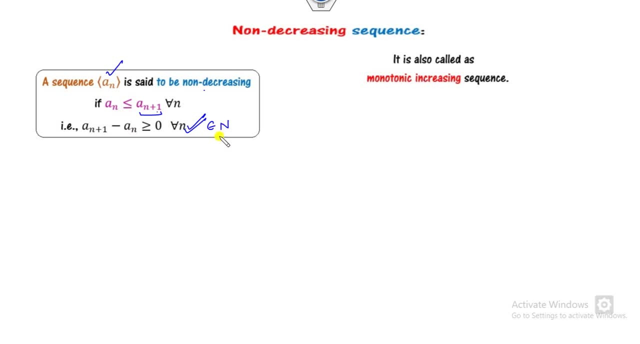 can say n is greater than 0 for all n in the domain natural number. Another definition is: we can say a sequence: an is said to be the non-decreasing if the ratio of the next term to the previous term is always greater than 1 for all n in the natural number. Similarly, if you look about this sequence, 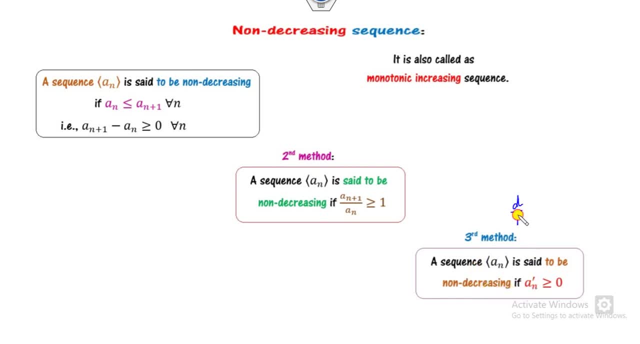 is said to be the non-increasing if the derivative of this sequence with respect to n is my greater than 0. Then we can say it is a increasing sequence. For example, if I try to check whether it is a non-decreasing or not, we will apply that all. 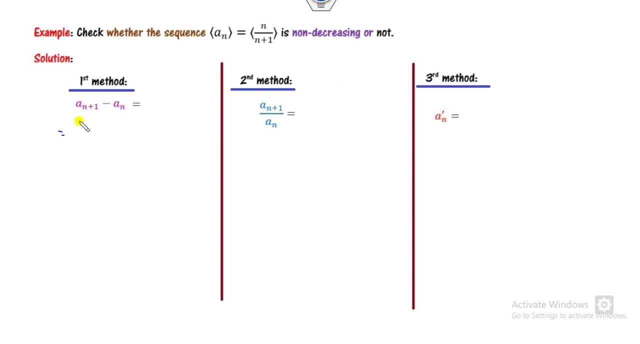 these three methods. What is the a n plus 1?? So you can see, a n plus 1 is nothing but n plus 1 upon n plus 2.. Now you can see: after the calculation you will get here, Can this number be always be? 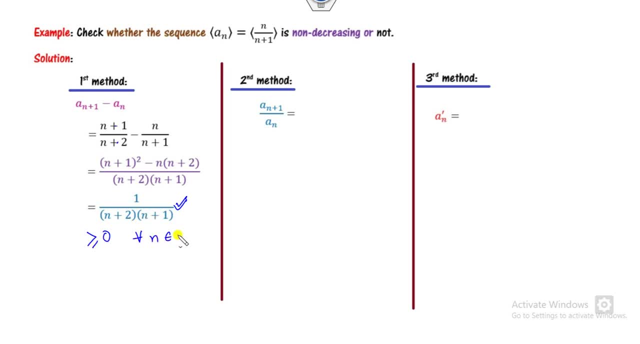 greater than or equal to 0? Yes, Why? Because n is my natural number and natural number is start from the 1,, 2,, 3.. So it is always positive. So this number is always positive. So you can say: 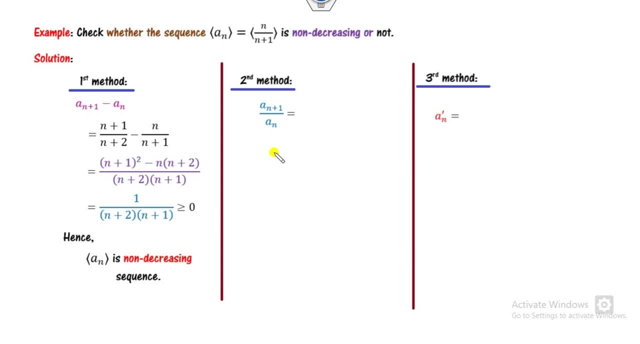 my. this is a non-decreasing sequence. Similarly, look about the second methods. What is the a n plus 1?? So if you look about that, this is my a n plus 1 over a n. So if you solve them, you will see these. 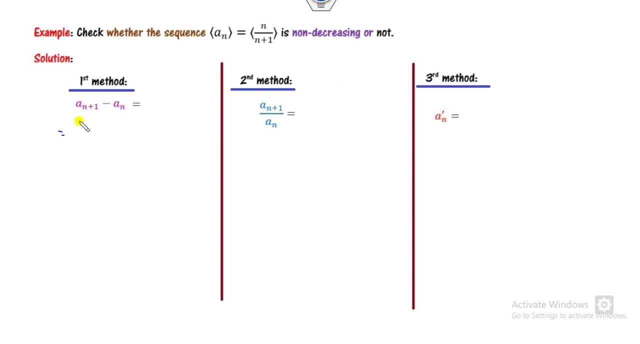 these three methods. What is the a n plus 1?? So you can see, a n plus 1 is nothing but n plus 1 upon n plus 2.. Now you can see: after the calculation you will get here, Can this number be always be? 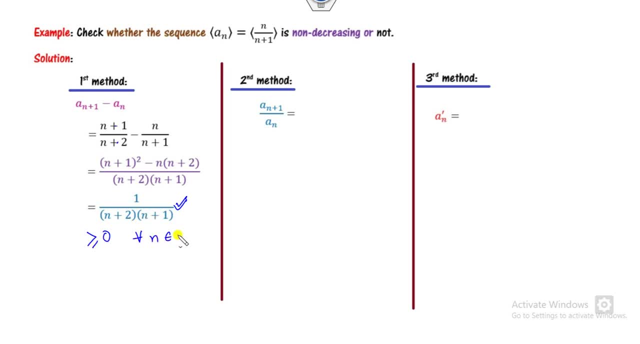 greater than or equal to 0? Yes, Why? Because n is my natural number and natural number is start from the 1,, 2,, 3.. So it is always positive. So this number is always positive. So you can say: 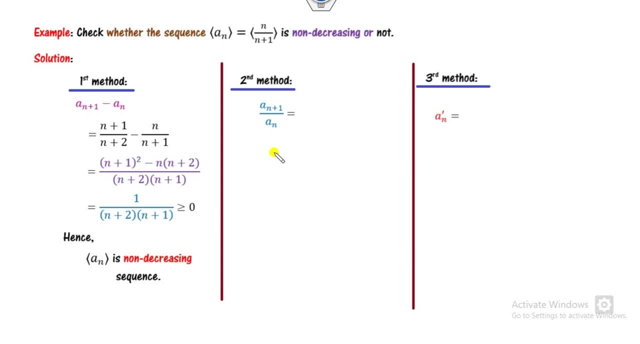 my. this is a non-decreasing sequence. Similarly, look about the second methods. What is the a n plus 1?? So if you look about that, this is my a n plus 1 over a n. So if you solve them, you will see these. 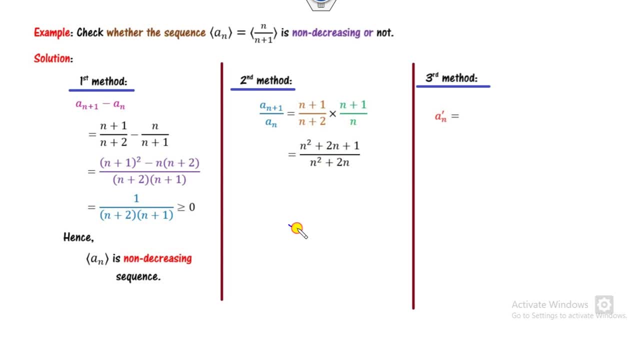 are my sequence. Now how you can say this number is my greater than 1?? So, if you see, I can return this number as 1 upon n square plus of 2n. Now you can see n is my natural number, which is always. 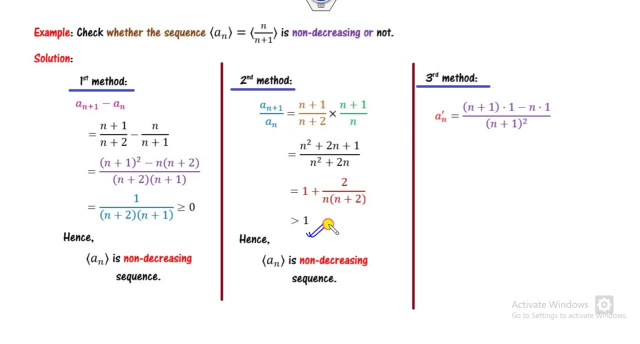 positive. So this number is always b Greater than 1.. Third method is: you can take the derivative of this. So what is the derivative of this? Here you can see again my. This number is, again you can see, always be greater than of the. 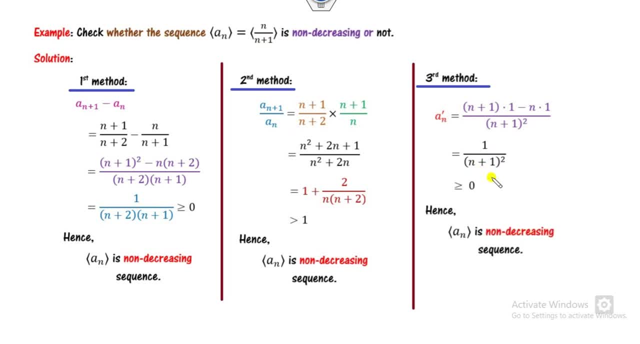 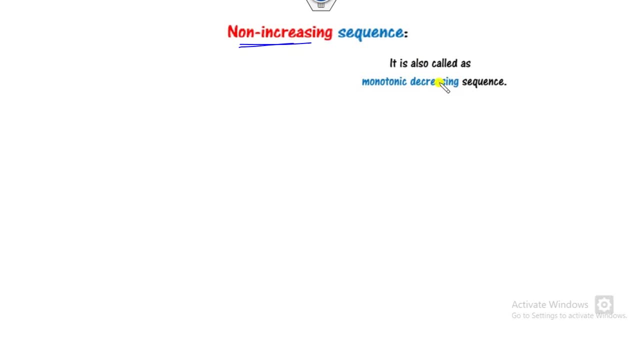 0, because this number can never be infinity. So it means it is a non-decreasing sequence. On the other hand, how you can see whether it is a non-increasing or you can say it is a decreasing sequence. So that is all. the results are reversed, That is a n plus 1 upon a n should. 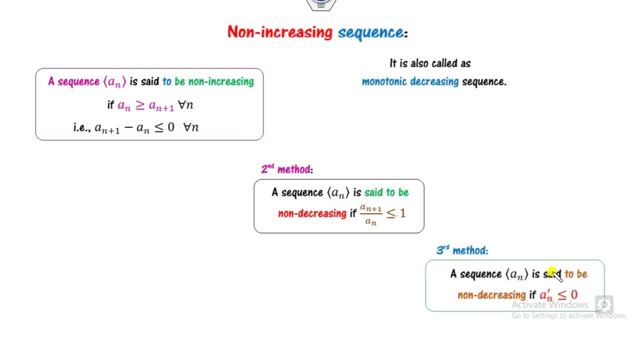 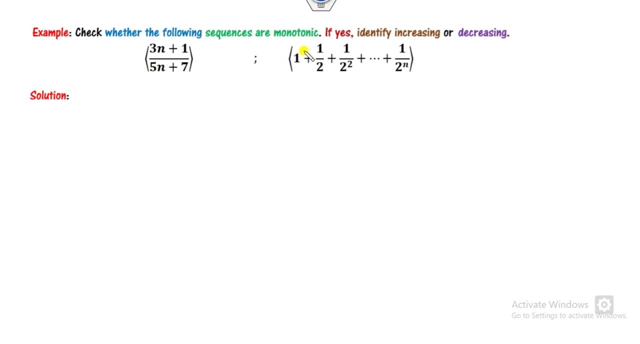 be greater than 1 and their derivative must be less than 0. So then you can say: the sequence are my decreasing sequence. So check which of the following sequence are my monotonic. If yes, check whether they are increasing or decreasing. So let us start with the first case. Again, we will apply. 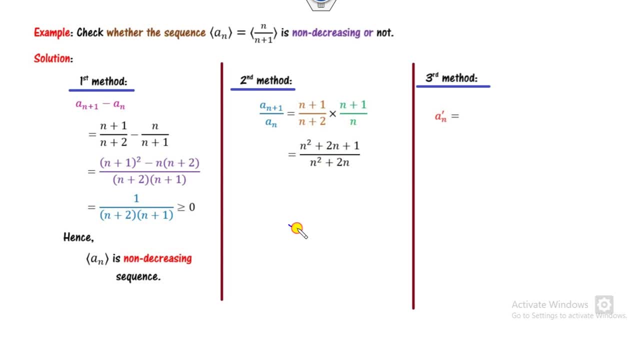 are my sequence. Now how you can say this number is my greater than 1?? So, if you see, I can return this number as 1 upon n square plus of 2n. Now you can see n is my natural number, which is always. 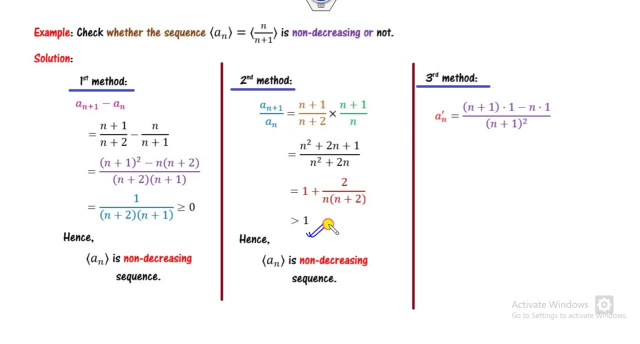 positive. So this number is always b Greater than 1.. Third method is: you can take the derivative of this. So what is the derivative of this? Here you can see again my. This number is, again you can see, always be greater than of the. 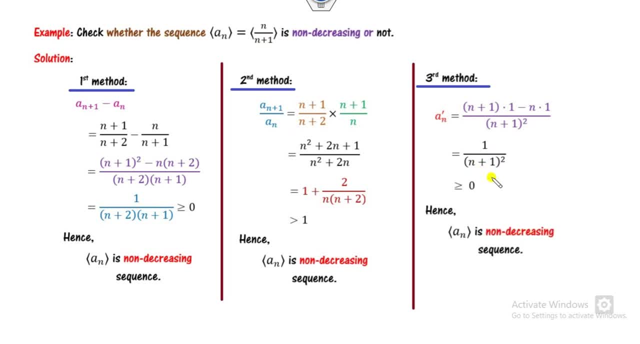 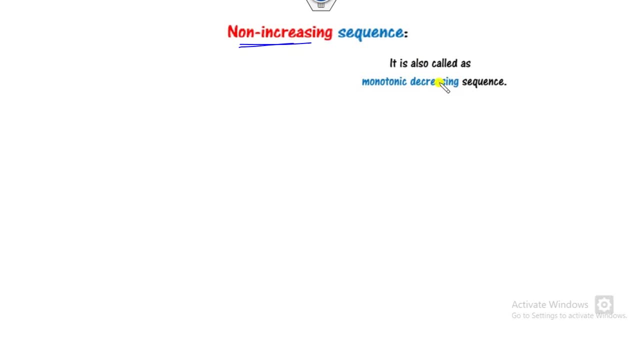 0, because this number can never be infinity. So it means it is a non-decreasing sequence. On the other hand, how you can see whether it is a non-increasing or you can say it is a decreasing sequence. So that is all. the results are reversed, That is a n plus 1 upon a n should. 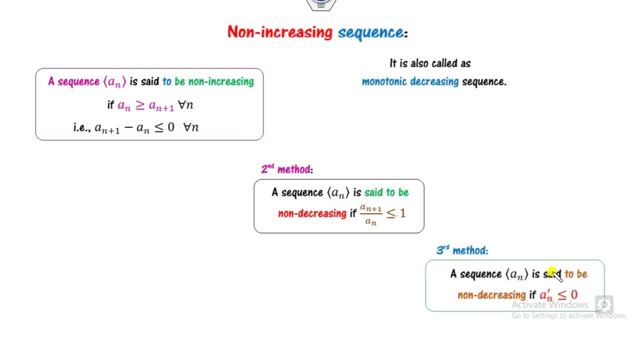 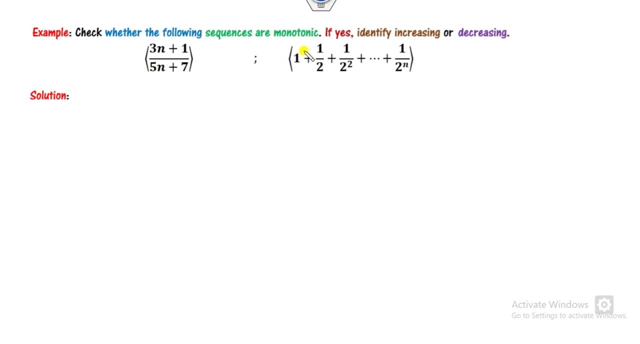 be greater than 1 and their derivative must be less than 0. So then you can say: the sequence are my decreasing sequence. So check which of the following sequence are my monotonic. If yes, check whether they are increasing or decreasing. So let us start with the first case. Again, we will apply. 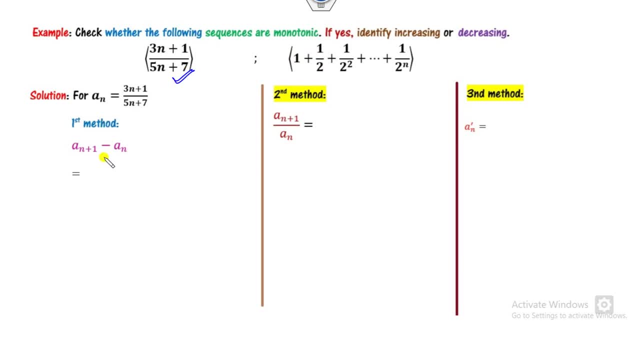 these three methods are here. The first method is here. You can check the. what is the a n plus 1.. You can say: this is a 3n plus 4 divided by 5n plus 12n minus. here You can take the LCM. Now you can open this bracket. You can see it is a 15n square, It will. 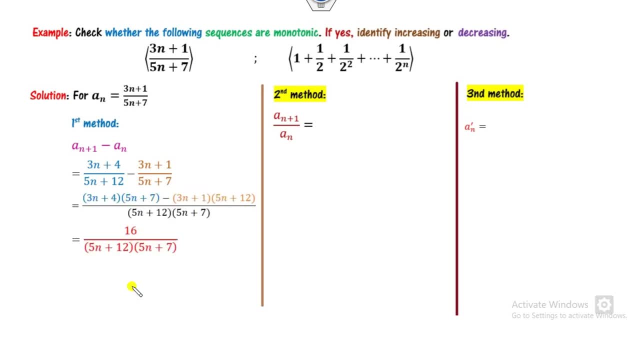 be cancelled out and so on. after the calculation you will get here. This number you always see, is a greater than or equal to 0, because for all n in the natural number. So it means it is a monotonically increasing sequence. Look for this one. So what is the a n plus 1 upon a n for this? 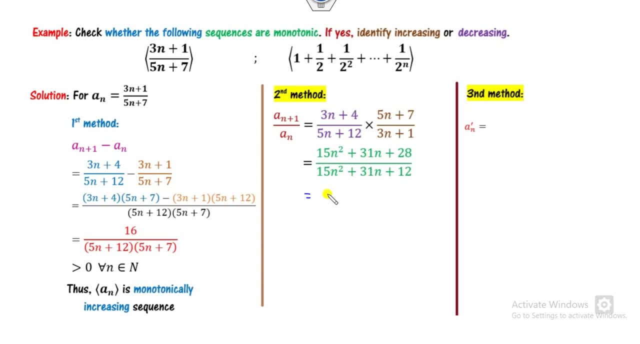 You can see this number is my here. Again, if you divide them you can easily see this number is my 16, over this denominator part. Again, this number is always be positive. So 1 plus something is always be greater than 1.. So it means this is again a monotonic increasing sequence. The third: 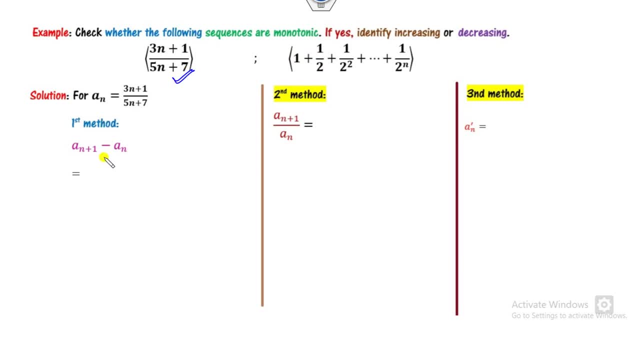 these three methods are here. The first method is here. You can check the. what is the a n plus 1.. You can say: this is a 3n plus 4 divided by 5n plus 12n minus. here You can take the LCM. Now you can open this bracket. You can see it is a 15n square, It will. 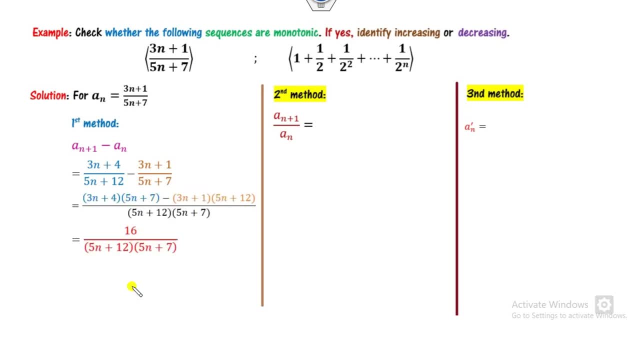 be cancelled out and so on. after the calculation you will get here. This number you always see, is a greater than or equal to 0, because for all n in the natural number. So it means it is a monotonically increasing sequence. Look for this one. So what is the a n plus 1 upon a n for this? 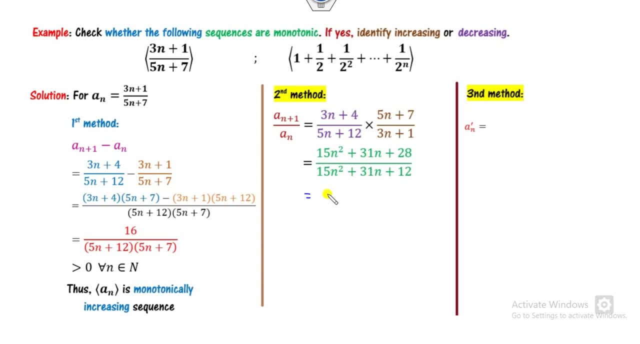 You can see this number is my here. Again, if you divide them you can easily see this number is my 16, over this denominator part. Again, this number is always be positive. So 1 plus something is always be greater than 1.. So it means this is again a monotonic increasing sequence. The third: 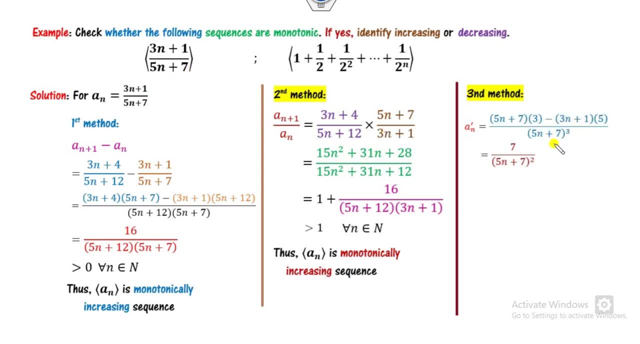 case you can take the derivative of this sequence. You can take the derivative as here Again you can see, this number is always be greater than 0 for all n in the natural number. So hence, by each of the method you can get a sequence is monotonically increasing sequence. 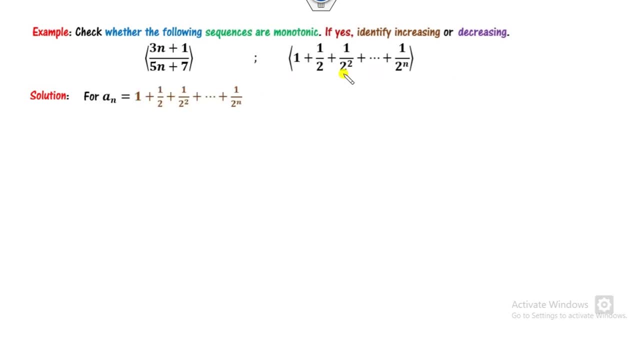 Look for the next example. So how you can see. So for this a n, we will try to find a n plus 1 minus of a n You will get here Clearly says that one will be cancelled out, Half will be cancelled out. 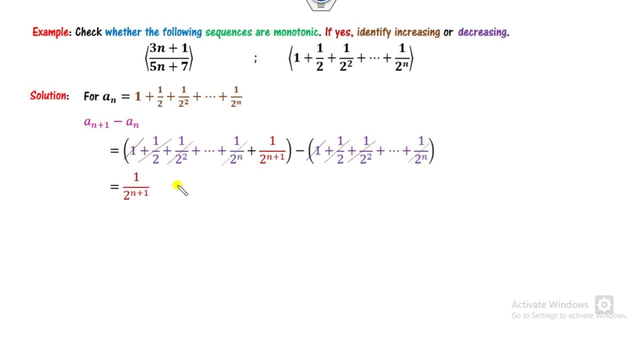 This will be cancelled out and the last one will be cancelled out. The only thing is my here, which is always be greater than 0 for all n in the natural number. So it therefore this sequence is a monotonic increasing sequence. You can apply the second method. 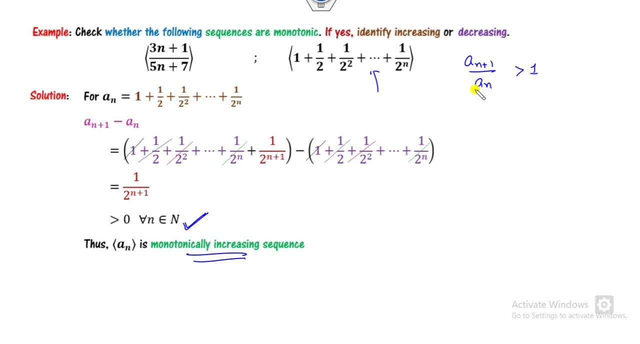 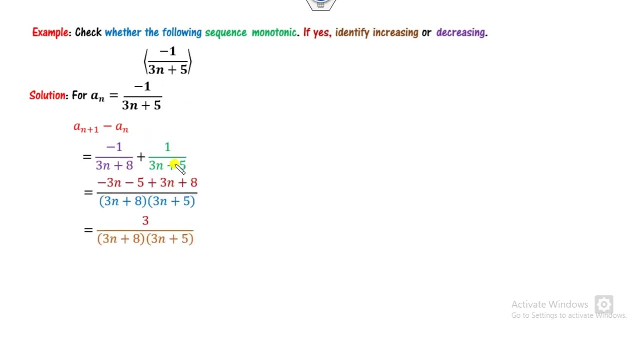 So if you want to find the ratio again, you will get as a greater than 1. But here you can't apply as a derivative of this. Look for the another one. Check whether it's a monotonic increasing or not. So again we will start with the first method. You can take the calcium. You can see this number is. 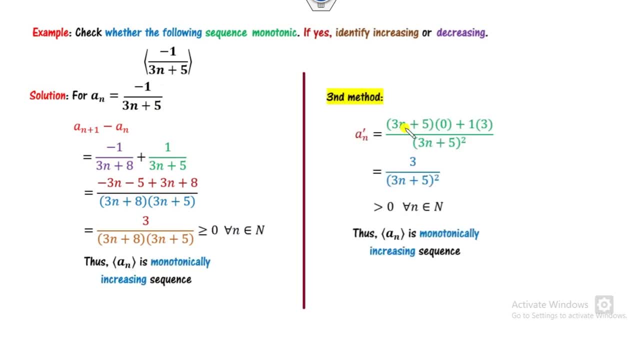 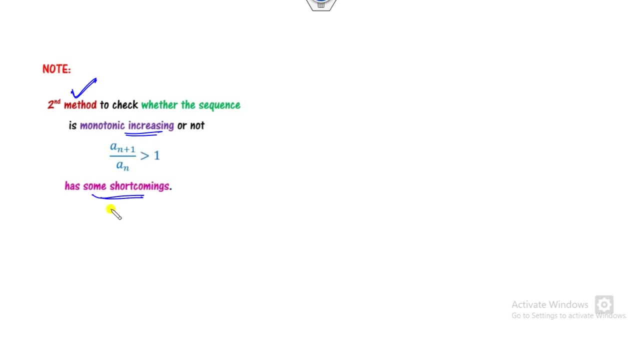 always be greater than 0. If you apply the third method here, because it's a derivative, So you can see here You should remember that the second method, that is a ratio is greater than 1 for the monotonic increasing, has some shortcomings, For example, if I consider the same example: 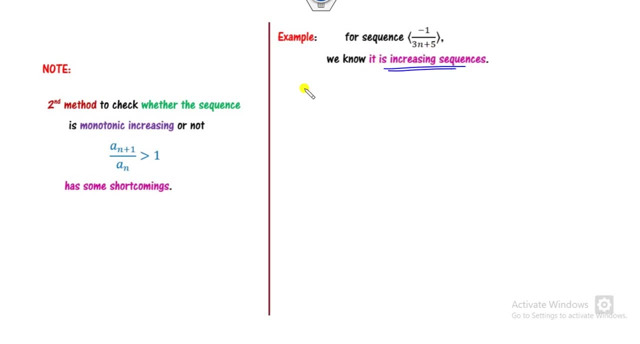 and we have discussed that it's increasing sequence. So what will happen if I compute a n plus 1 upon a n? So you can see this number is 1 minus of this. So this number is always positive, So is less than 0.. So what is the meaning of that? This is my decreasing sequence, but which? 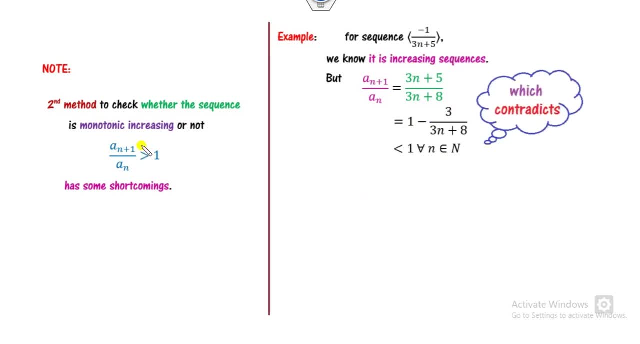 contradict about this factor. So it means this second method will not always give you the right answer. However, if you consider the sequence instead of the positive, you can clearly say that it is a decreasing sequence. Why? If you take the derivative, it will give you my here and you. 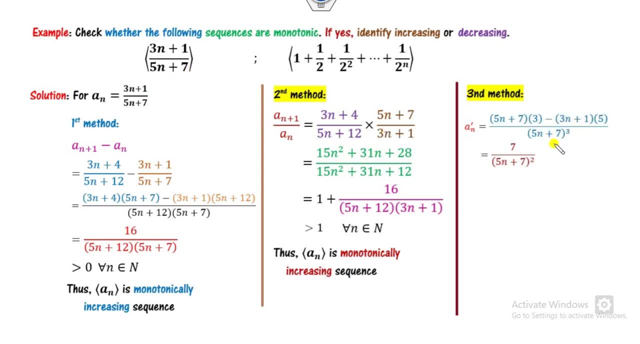 case you can take the derivative of this sequence. You can take the derivative as here Again you can see, this number is always be greater than 0 for all n in the natural number. So hence, by each of the method you can get a sequence is monotonically increasing sequence. 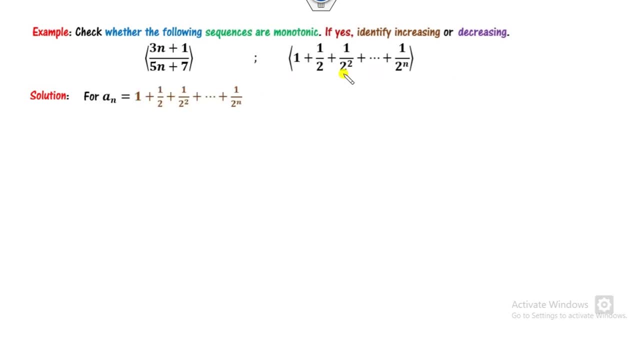 Look for the next example. So how you can see. So for this a n, we will try to find a n plus 1 minus of a n You will get here Clearly says that one will be cancelled out, Half will be cancelled out. 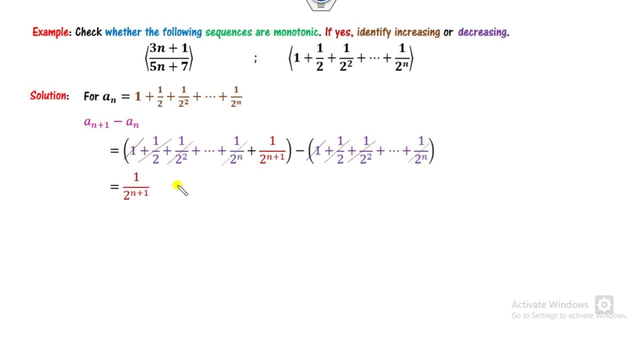 This will be cancelled out and the last one will be cancelled out. The only thing is my here, which is always be greater than 0 for all n in the natural number. So it therefore this sequence is a monotonic increasing sequence. You can apply the second method. 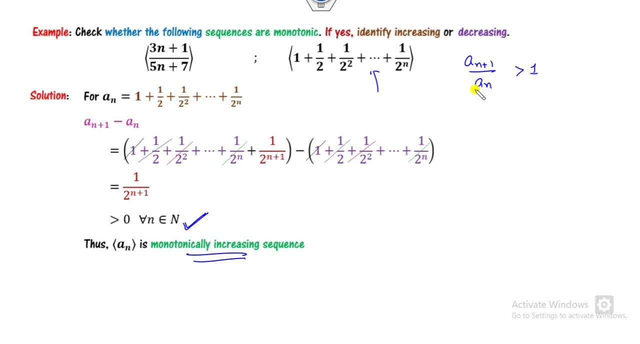 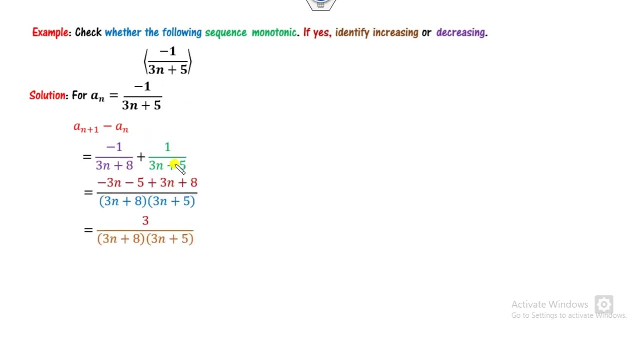 So if you want to find the ratio again, you will get as a greater than 1. But here you can't apply as a derivative of this. Look for the another one. Check whether it's a monotonic increasing or not. So again we will start with the first method. You can take the calcium. You can see this number is. 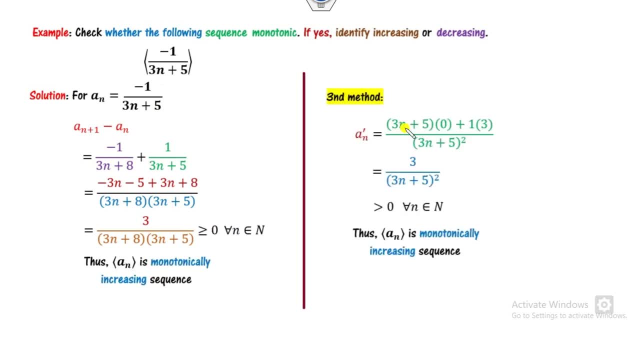 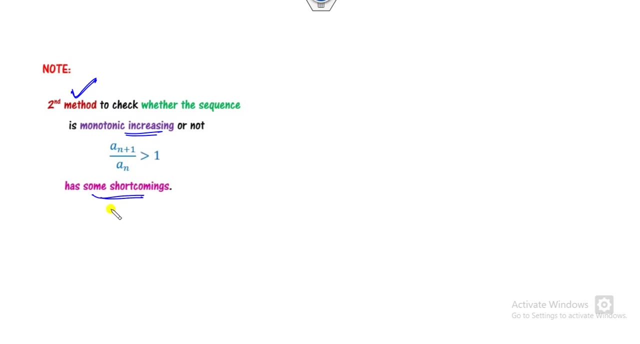 always be greater than 0. If you apply the third method here, because it's a derivative, So you can see here you should remember that the second method, that's a ratio, is greater than 1 for the monotonic increasing, has some shortcomings. For example, if I consider the same example and we have discussed 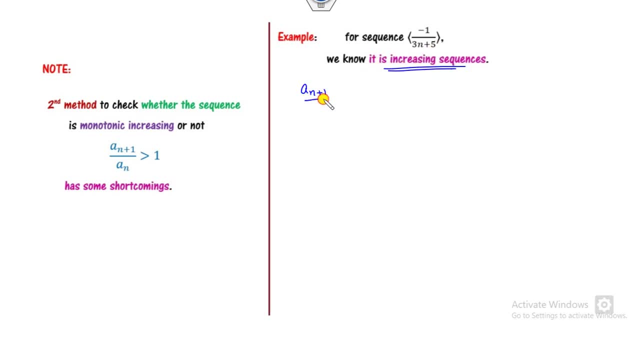 that it's increasing sequence. So what will happen if I compute a n plus 1 upon a n? So you can see this number is 1 minus of this. So this number is always positive, So is less than 0.. So what is the? 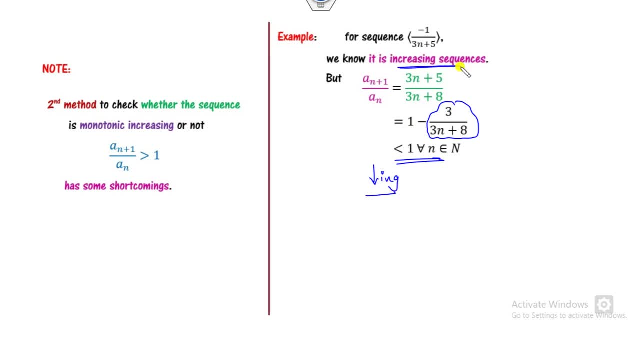 meaning of that. This is my decreasing sequence, but which contradict about this. So if you look at this factor, So it means this second method will not always give you the right answer. However, if you consider the sequence instead of the positive, you can clearly say that it is a. 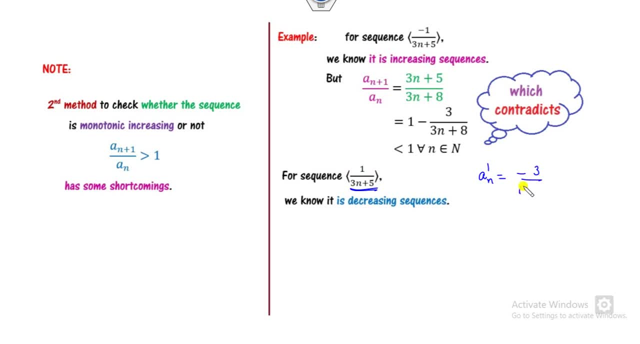 decreasing sequence. Why? If you take the derivative, it will give you my here and you can see this is always be less than 0. So it means it is a decreasing. So if you try to solve this again, you will get as a decreasing sequence. So what is the meaning of that? If you consider, 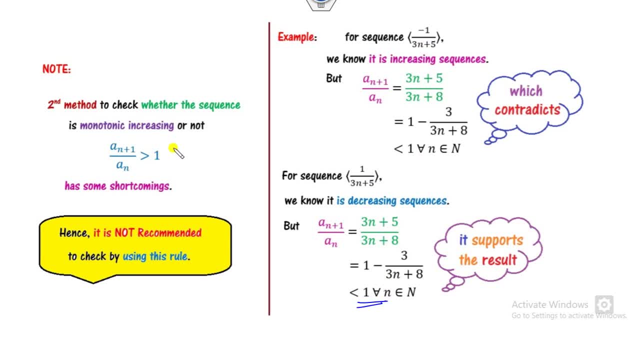 the same number. one is a negative, one is a positive. that will not distinguish by the second method. So therefore, I recommend not to use this method to check whether it is increasing or decreasing. So you always try to check whether it is increasing or decreasing by using this one. 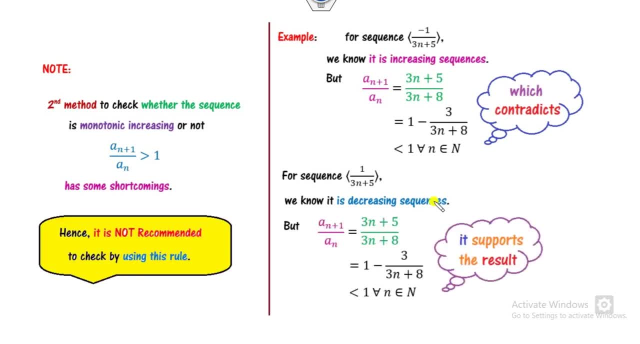 can see, this is always be less than 0. So it means it is a decreasing. So if you try to solve this again, you will get as a decreasing sequence. So what is the meaning of that? If you consider the same number, one is a negative, one is a positive. that will not distinguish by the. 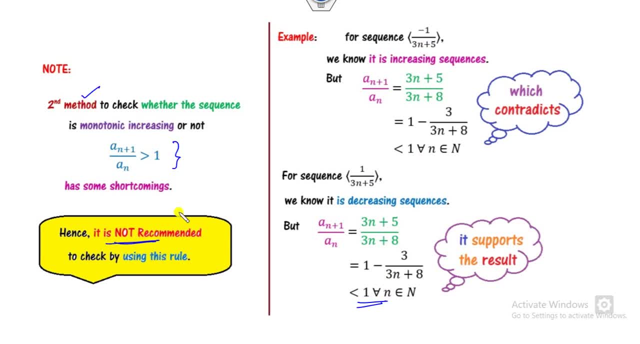 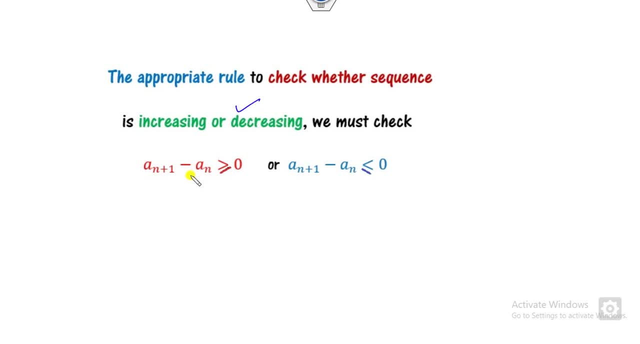 second method. So therefore I recommend not to use this method to check whether it is increasing or decreasing. So you always try to check whether it is increasing or decreasing by using this one. So if this condition satisfied, we call it as increasing. Otherwise, this condition satisfied. 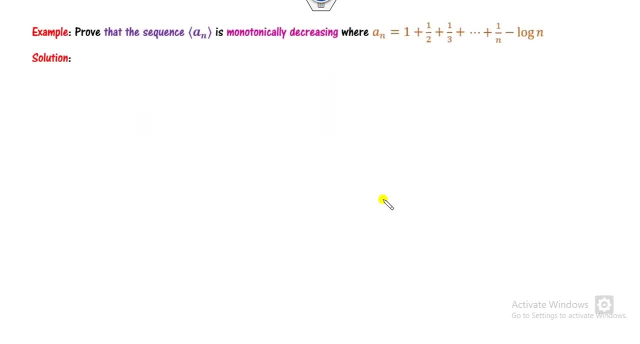 we call as a decreasing sequence. Look at this. Some more examples are there. We will try to cover the 15 examples in this video so that you may be able to understand more clearly. So if a n is my, this sequence, you can compute the a n plus 1.. Your target is to prove that a n plus 1 minus of a n. 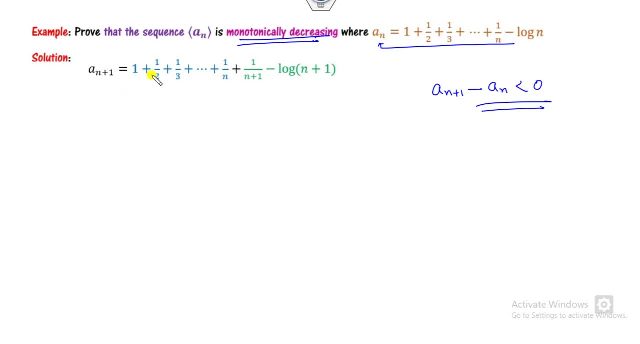 should be less than 0. This is your target because of the decreasing, Now you can find the a n plus 1 minus a n. If you subtract them, you can see up to this will be cancelled and the remaining part- here I can combine them You will get. here I can apply the. 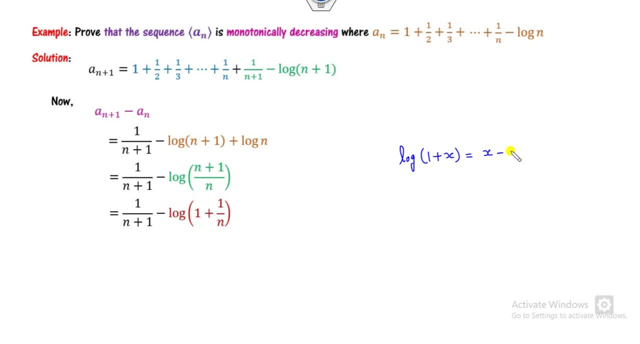 logarithm series log of the 1 plus x. It is nothing but x minus x square upon 2 plus and so on. We can apply like here: I can open this bracket and take the pair of this. You can clearly say that this number is my positive because if you take the LCM it will be give you 4 n minus 3 over. 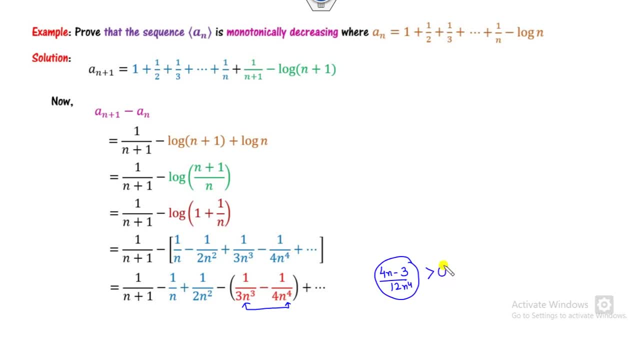 12 and 4.. It is always be a greater than 0 because n is my natural number, So it means this number is positive. If I consider this as number and this is negative, it means this number is less than of here. because of this negative. If you take the LCM of this. 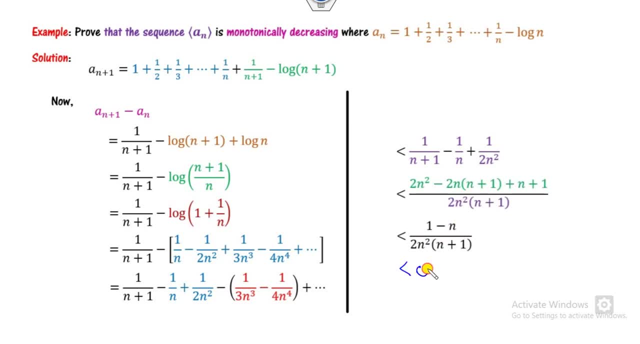 you will get here. So can you say this number is always be less than 0? Yes, because it is a 1 minus n. This denominator part is always positive, but this is always negative, for all n belongs to the natural number, So it is a less than or equal to 0. Hence it is a monotonic, decreasing sequence. 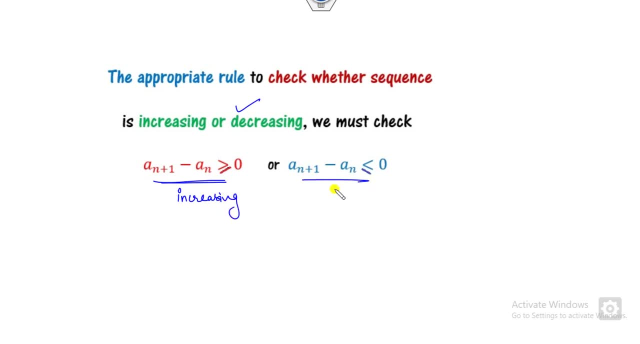 So if this condition satisfied, we call it as increasing. Otherwise, this condition satisfied, we call as a decreasing sequence. Look at this. Some more examples are there. We will try to cover the 15 examples in this video so that you may be able to understand more clearly. So if a n is my, this: 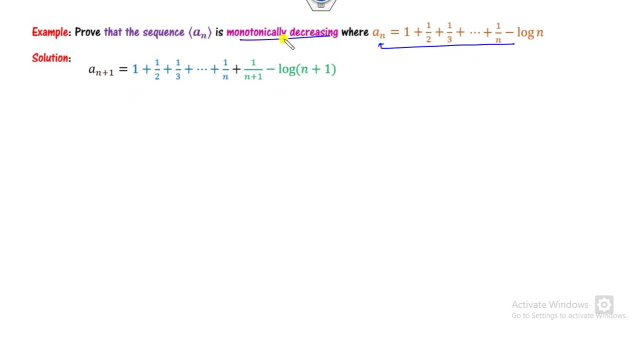 sequence, you can compute the a n plus 1.. Your target is to prove that a n plus 1 minus of a n should be less than 0. This is your target. because of the decreasing, Now you can find the a n plus. 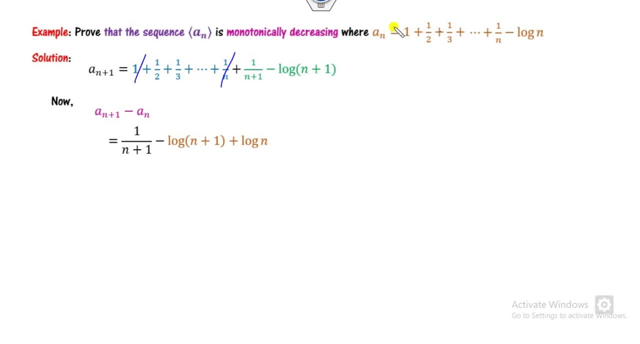 1 minus a n- If you subtract them you can see up to this- will be cancelled, and the remaining part- here I can combine them, You will get here I can apply the logarithm series log of the 1 plus x. It is nothing but x minus, x square upon 2 plus, and so 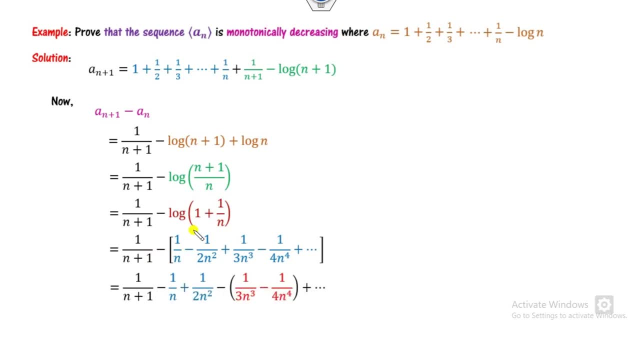 on. We can apply like here. I can open this bracket and take the pair of this. You can clearly say that this number is my positive because if you take the LCM it will be: give you 4, n minus 3 over 12 and 4.. It is always be a greater than 0 because n is my natural number, So it means this number. 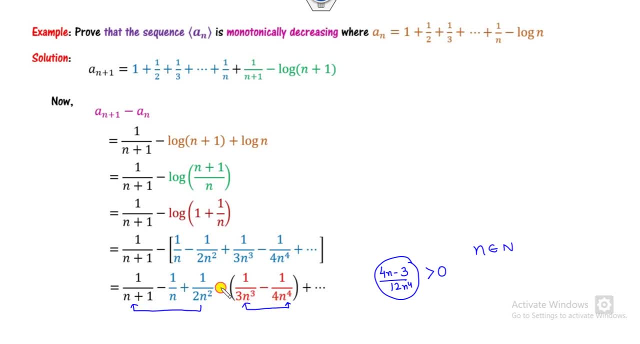 is positive. If I consider this as number and this is negative, it means this number is less than of here. because of this negative, If you take the LCM of this, you will get here. So can you say this number is always be less than 0?? Yes, because it is a 1. 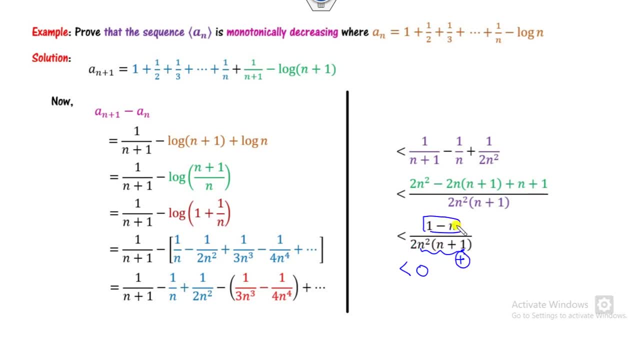 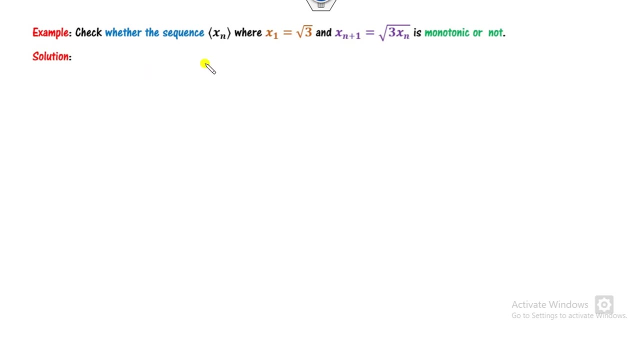 minus n. This denominator part is always positive, but this is always negative, for all n belongs to the natural number, So it is a less than or equal to 0. Hence it is a monotonic decreasing sequence. Look for the second type part there How you can. 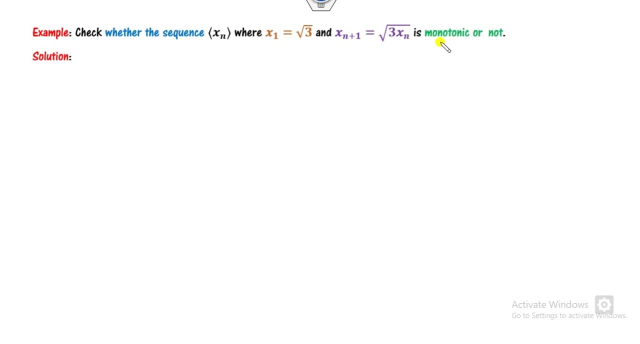 check whether the sequence is monotonic or not. Here your target is to check whether it is a monotonic increasing or decreasing. It means your target is to check whether this happen or this happen. So let us firstly check whether this happens or not. So we will try to solve this. 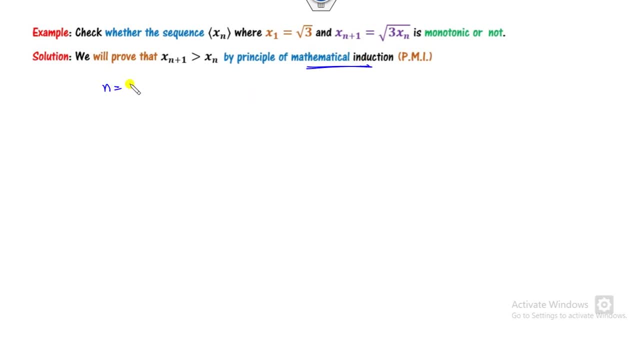 with the help of mathematical induction. So what will we do? We can start with. n is equal to 1.. So what is the value of this? So x2.. x2 is nothing but my. here We know the value of the x1. I can substitute this value. So clearly says that this number 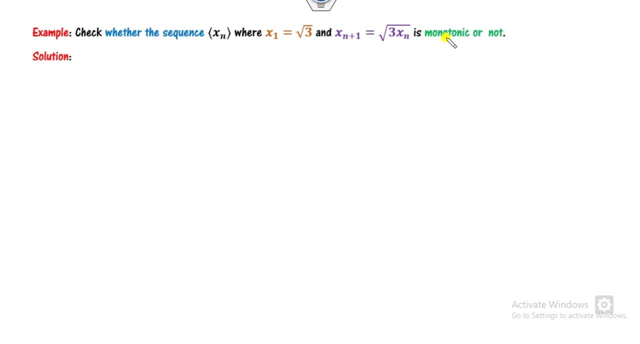 Look for the second type part there, How you can check whether the sequence is monotonic or not. Here your target is to check whether it is a monotonic increasing or decreasing. It means your target is to check whether this happen or this happen. So let us firstly check whether this happens or not. So we will try to solve this. 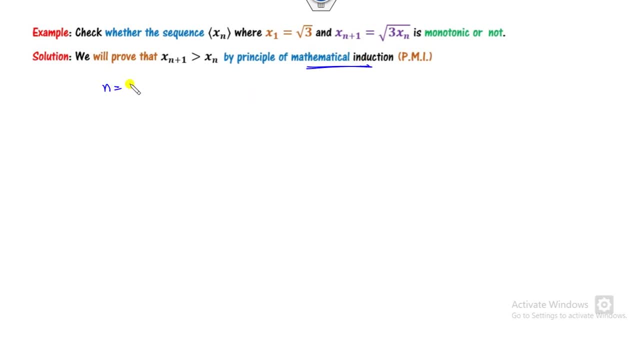 with the help of mathematical induction. So what will we do? We can start with. n is equal to 1.. So what is the value of this? So x2.. x2 is nothing but my. here We know the value of the x1. I can substitute this value. So clearly says that this number 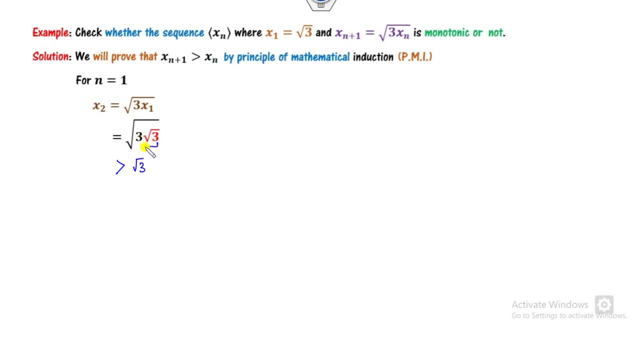 is greater than of root 3, because its answer is: So what is the x3?? It is my x1. So x2 is greater than x1. It means the result is 2 for n is 1.. Assume that the result is 2 for n is equal to k. 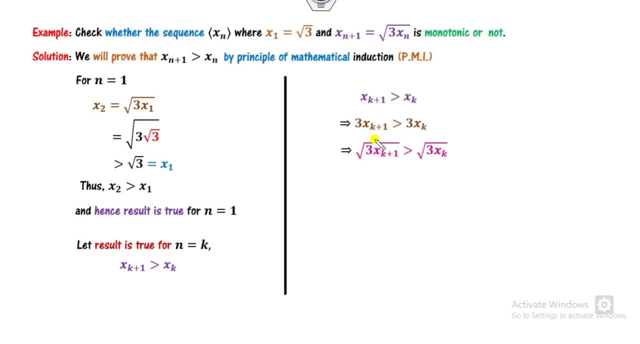 Then we can simply multiply by 3 on the both side. Take the square root p. What will happen? This is nothing but x plus 2.. This is xk plus 1.. So therefore, the result is true, for all the n belongs to the natural Hence. 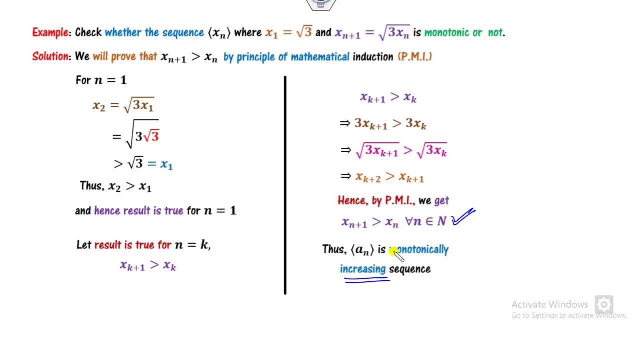 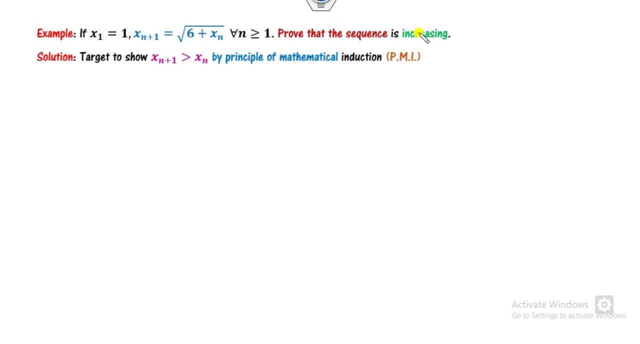 the sequence is monotonic, increasing. Look at the similar kind of the second example. So whether it is increasing. So your target is to prove that it is an increasing sequence. Again, we apply the principle of mathematical induction. If you take n is 1, it is my x2.. 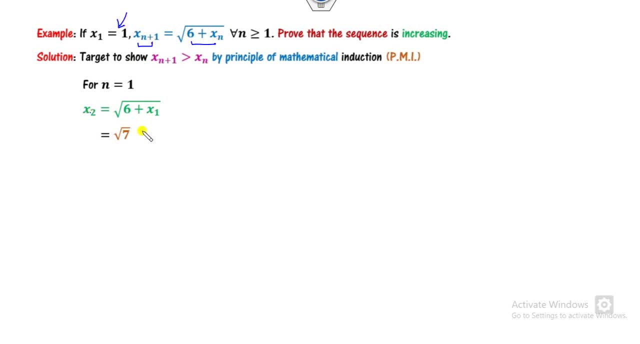 This is 6 plus x1.. x1 is given to be here, So can it be greater than of the x1?? What is x1?? It is a 1.. So this number is always be greater than of the 1, because root 7 is. What is the root 7?? It is a 2 point, something. It is greater than 1.. Hence, 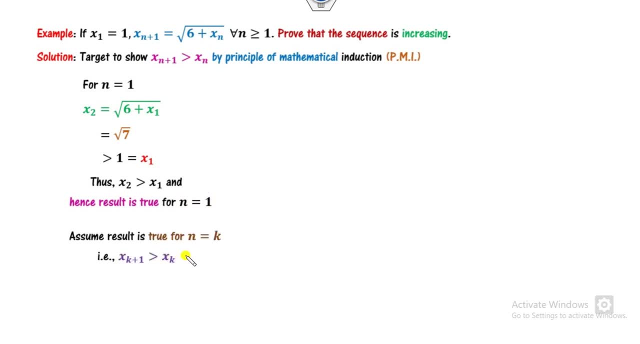 result is 2 for here, Assume the result is 2, for n is equal to k. Now I need a 6 plus something So I can add in the 6 on the both side and then take the square root of this. So what will happen? 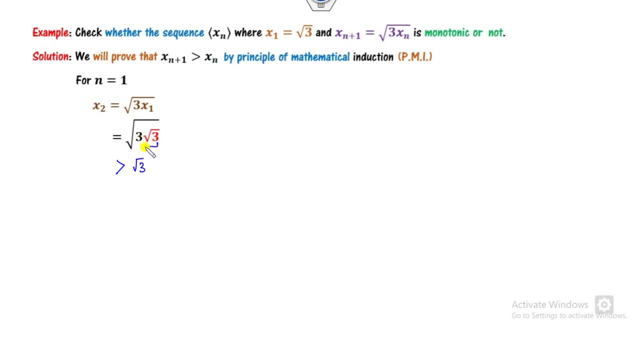 is greater than of root 3, because its answer is: So what is the x3?? It is my x1. So x2 is greater than x1. It means the result is 2 for n is 1.. Assume that the result is 2 for n is equal to k. 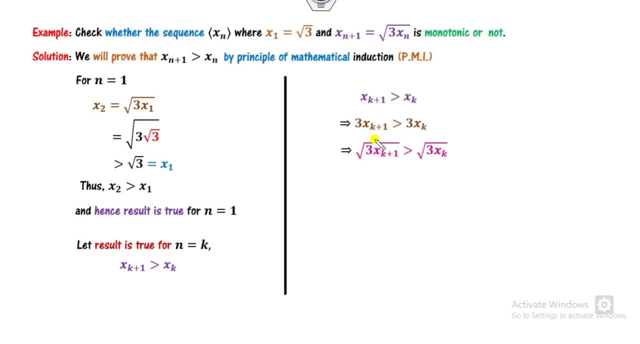 Then we can simply multiply by 3 on the both side. Take the square root p. What will happen? This is nothing but x plus 2.. This is xk plus 1.. So therefore, the result is true, for all the n belongs to the natural Hence. 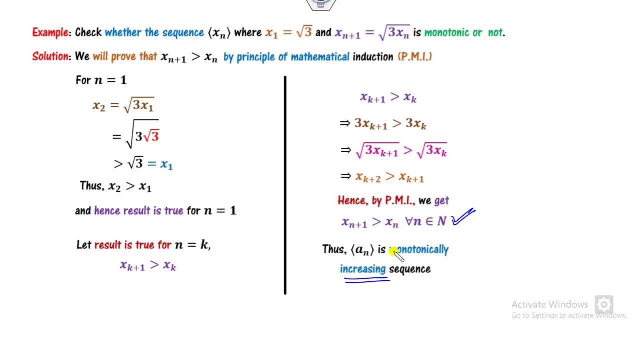 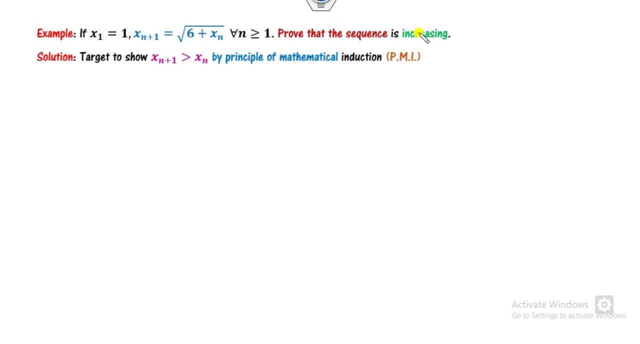 the sequence is monotonic, increasing. Look at the similar kind of the second example. So whether it is increasing. So your target is to prove that it is an increasing sequence. Again, we apply the principle of mathematical induction. If you take n is 1, it is my x2.. 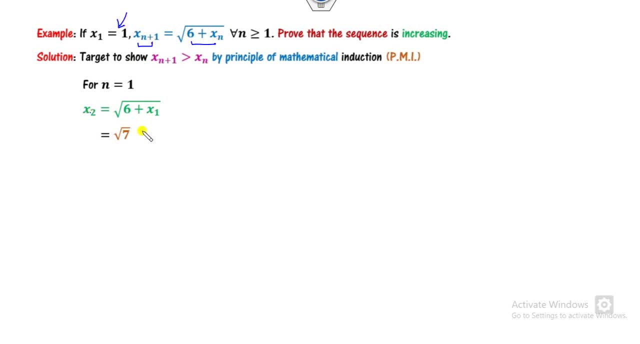 This is 6 plus x1.. x1 is given to be here, So can it be greater than of the x1?? What is x1?? It is a 1.. So this number is always be greater than of the 1, because root 7 is. What is the root 7?? It is a 2 point, something. It is greater than 1.. Hence, 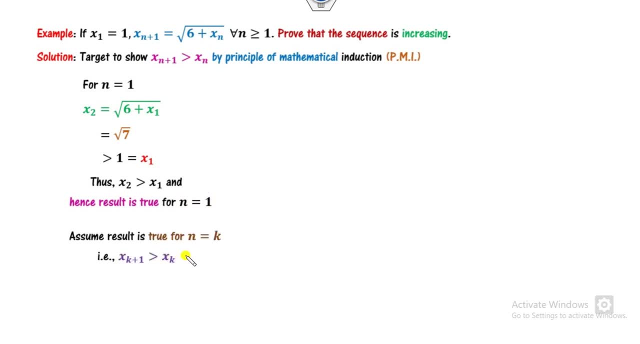 result is 2 for here, Assume the result is 2, for n is equal to k. Now I need a 6 plus something So I can add in the 6 on the both side and then take the square root of this. So what will happen? 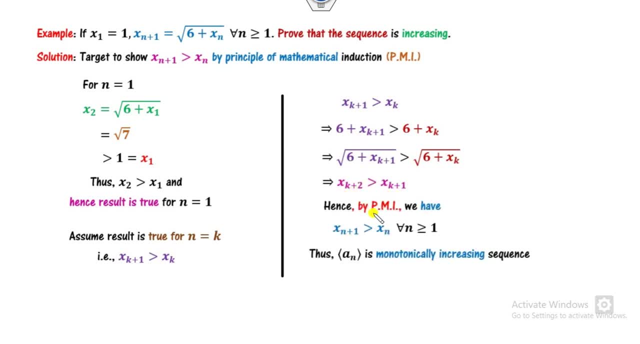 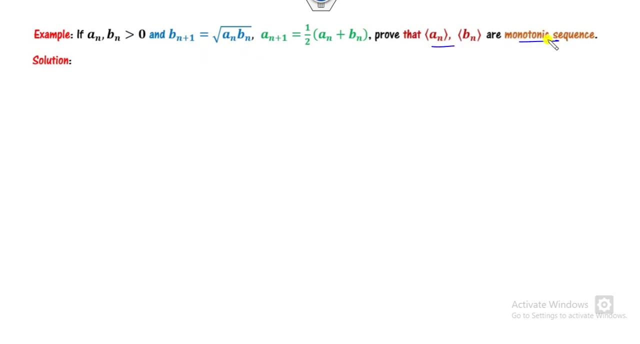 This is my here. So therefore, by the principle of the mathematical induction, the result is 2, for this n belongs to the natural, Hence it is a monotonic increasing sequence. Now look at the third kinds are there. So in this case, your target is to check what is the nature of the 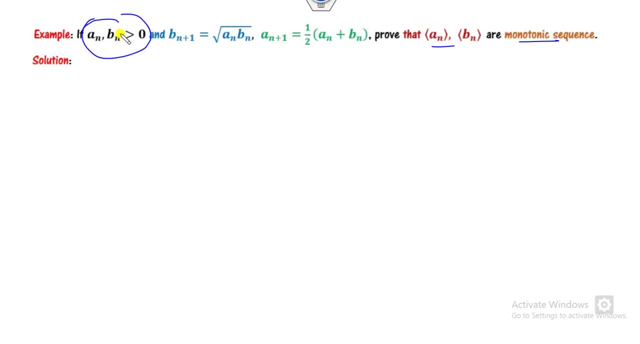 sequence. It is given that both the a? n is greater than 0, b? n is greater than 0. But they are not talking about that. whether a? n is this or a n is less than of this. This is not given to you, So. 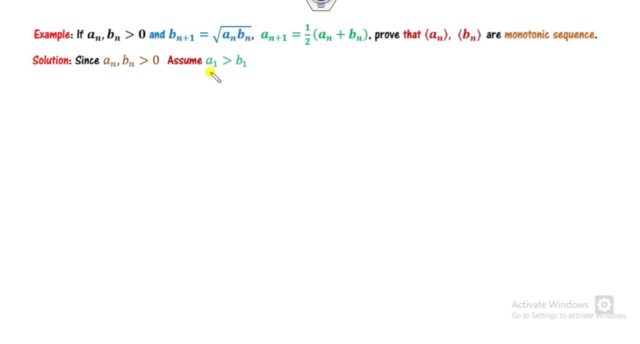 what we can do. I assume that b n is greater than 0. So what we can do. I assume that b n is greater than 0. So what we can do. I assume that a 1 is greater than of the b 1.. You may assume that a 1 is. 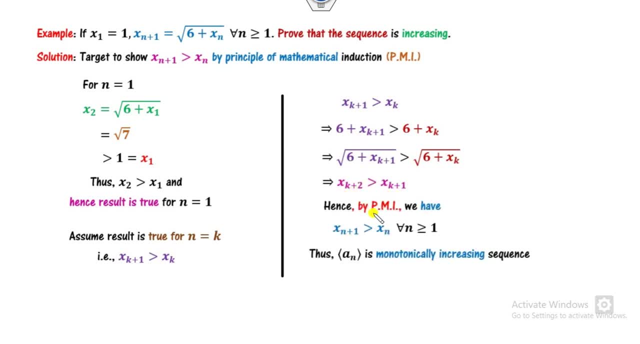 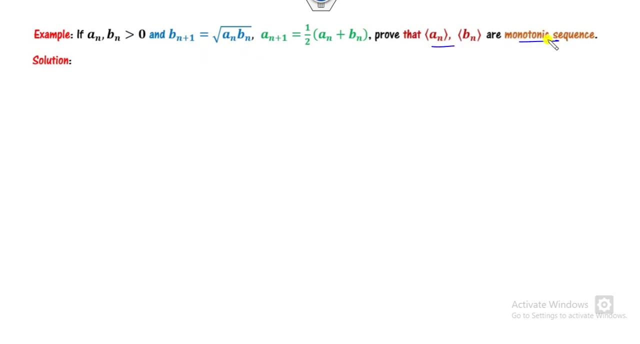 This is my here. So therefore, by the principle of the mathematical induction, the result is 2, for this n belongs to the natural, Hence it is a monotonic increasing sequence. Now look at the third kinds are there. So in this case, your target is to check what is the nature of the 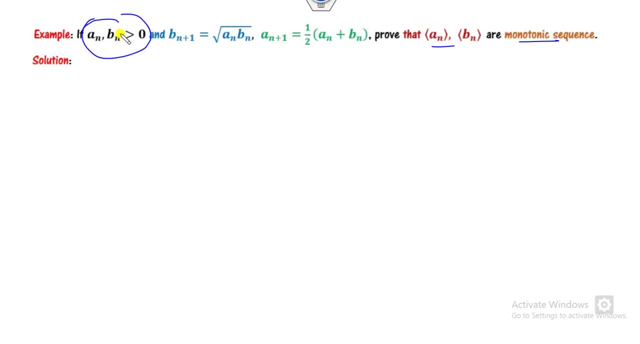 sequence. It is given that both the a? n is greater than 0, b? n is greater than 0. But they are not talking about that. whether a? n is this or a n is less than of this. This is not given to you, So. 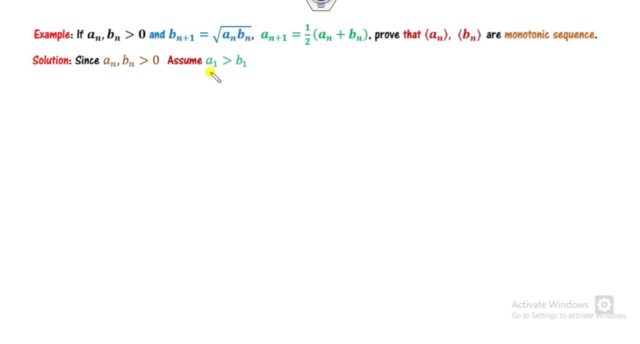 what we can do. I assume that b n is greater than 0. So what we can do. I assume that b n is greater than 0. So what we can do. I assume that a 1 is greater than of the b 1.. You may assume that a 1 is. 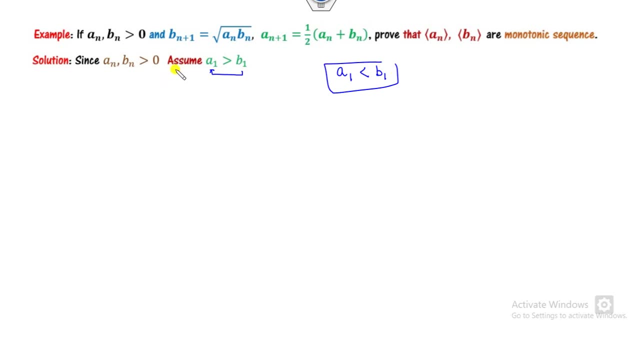 less than b 1.. It is on your choice, So let us start with this. So, firstly, we can take: n is 1.. So what will happen? It is my nothing, but b 2 is root of this. What is the meaning of that? It is: 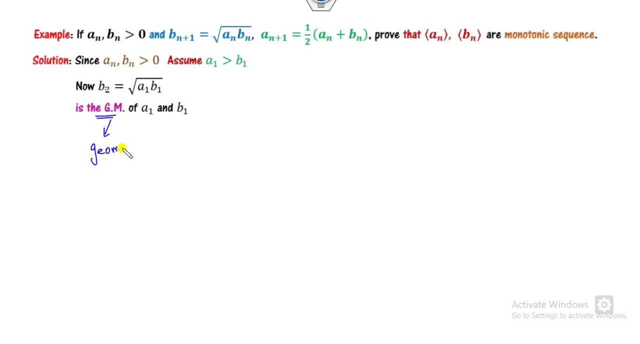 a geometric mean. This is called as geometric mean, So we know that if it is a geometric means, it means this: b 2 must lies in between them, And we know a 1 is greater than of the b 1.. So I can write as b 1.. Here is a 1 and b 2 lies between. 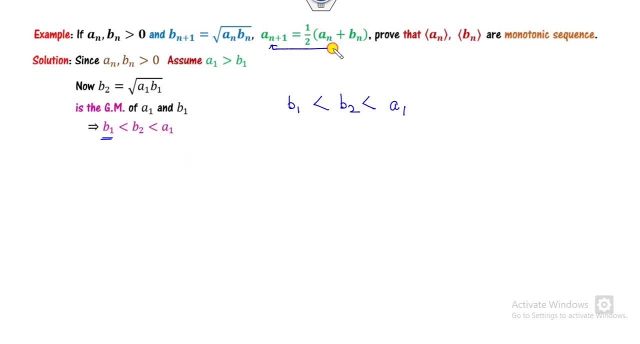 them in this manner. Similarly, I can substitute here We will get: as n is 1, it is a 2. It is a arithmetic mean, So a 1 and b 1.. So a 1 is bigger than of this, So a 2 lies in between them. 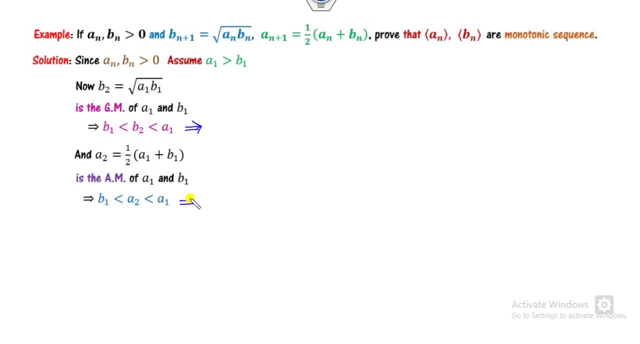 This is the sequence. So from here and from this I can say b 1 is less than b 2, but b 1 is less than a 2 also. So it means our target is to find the relation between them. So what is the b 2?? b 2 is the geometric mean. 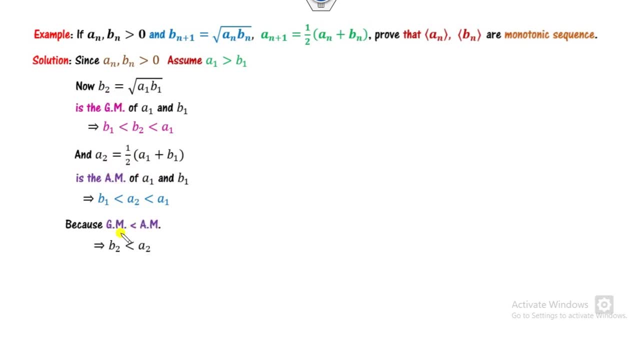 a 2 is the arithmetic mean. What is the relation between them? We all know about here. So, from this and from this, what you conclude? that b 1 is less than b 2, b 2 is less than a 2, a 2 is less. 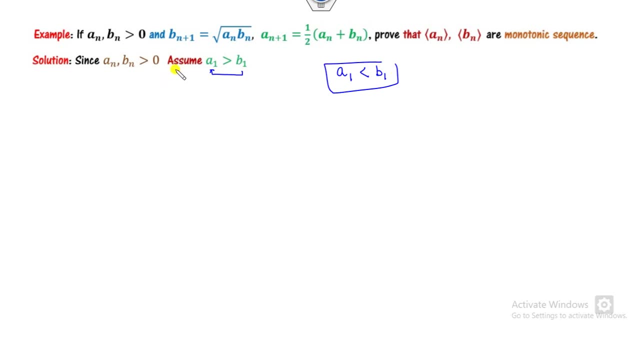 less than b 1.. It is on your choice, So let us start with this. So, firstly, we can take: n is 1.. So what will happen? It is my nothing, but b 2 is root of this. What is the meaning of that? It is: 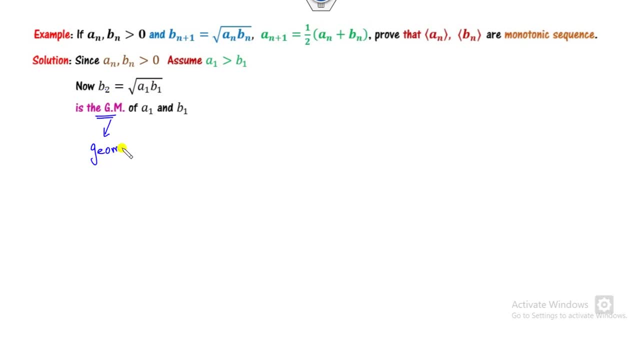 a geometric mean. This is called as geometric mean, So we know that if it is a geometric means, it means this: b 2 must lies in between them, And we know a 1 is greater than of the b 1.. So I can write as b 1.. Here is a 1 and b 2 lies between. 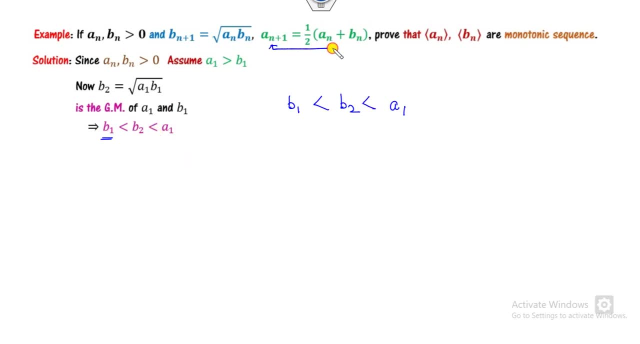 them in this manner. Similarly, I can substitute here We will get: as n is 1, it means a 2. It is arithmetic mean. So a 1 and b 1.. So a 1 is bigger than of this. So a 2 lies in between them. 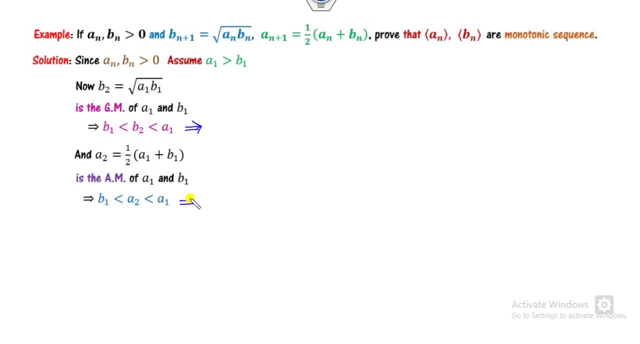 This is a sequence. So from here and from this I can say b 1 is less than b 2, but b 1 is less than a 2 also. So it means our target is to find the relation between them. So what is a b 2?? b 2 is a geometric mean. 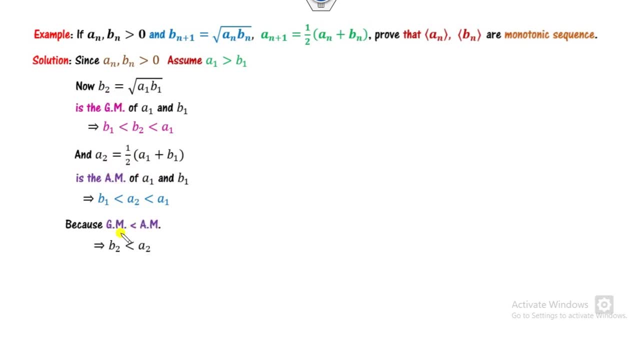 a 2 is arithmetic mean. What is the relation between them We all know about here. So, from this and from this, what you conclude? that b 1 is less than b 2, b 2 is less than a 2, a 2 is less. 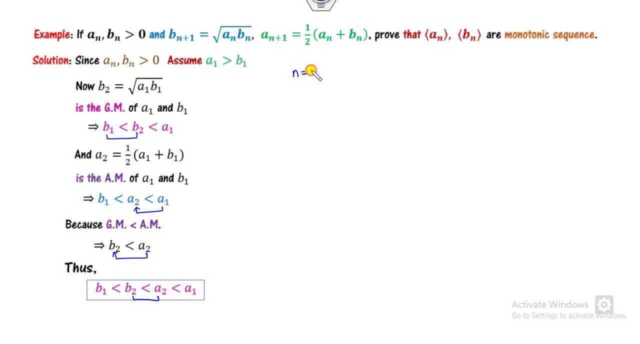 than a. Similarly, if you take n is equal to 2,. if you can calculate here, it is my b 3.. b 3 is nothing but a, 2, b 2.. What is the meaning of that? It means b 3 is the geometric mean of this, And what is the relation? 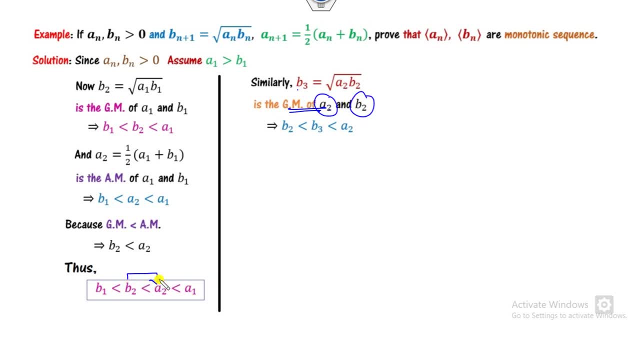 between a 2 and b 2?? We can see here a 2 is less than of the b 2. So b 3 lies between them. Similarly, from here Hence, arithmetic mean is always bigger than of the geometric mean. So from these three, 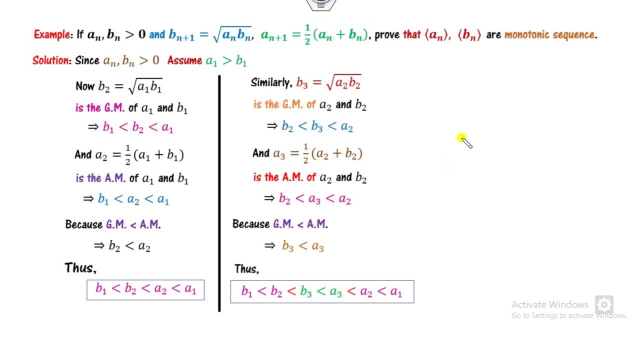 we can get as of here. So, similarly, if you extend them, what will happen? b 1 less than b, 2 less than b 3, and so on. Here is a 1 and so on. So what is the meaning of that? You can see b i. 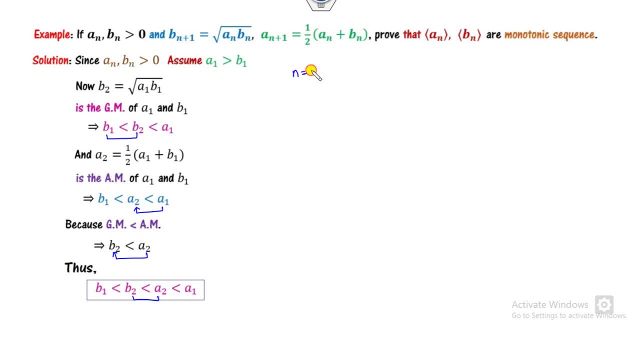 than a. Similarly, if you take n is equal to 2,. if you can calculate here, it is my b 3.. b 3 is nothing but a, 2, b 2.. What is the meaning of that? It means b 3 is the geometric mean of this, And what is? 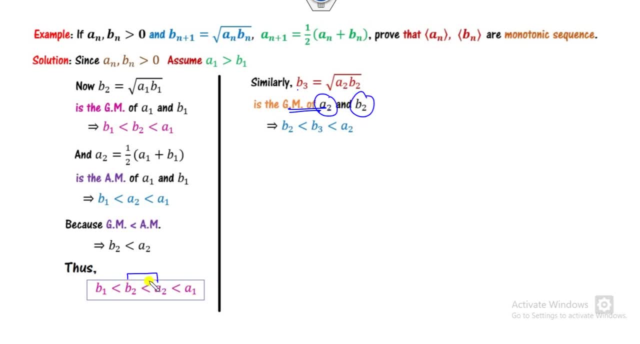 the relation between a 2 and b 2?. We can see here: a 2 is less than of the b 2. So b 3 lies between them Similarly from here. Hence arithmetic mean is always bigger than of the geometric mean. So 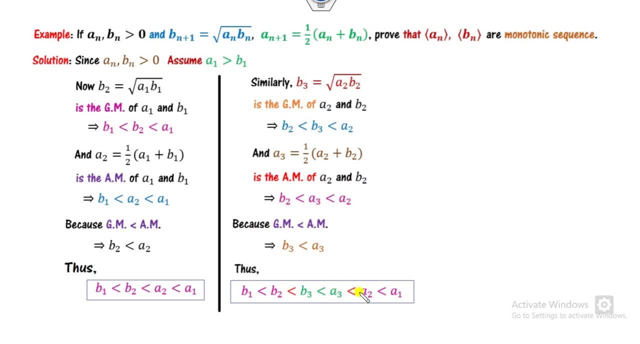 from these three relations we can get as of here. So, similarly, if you extend them, what will happen? b 1 less than b 2 less than b 3, and so on. Here is a 1 and so on. So what is the meaning of that? You can see b i. 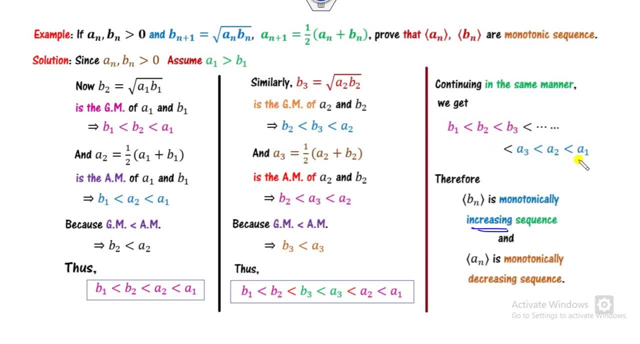 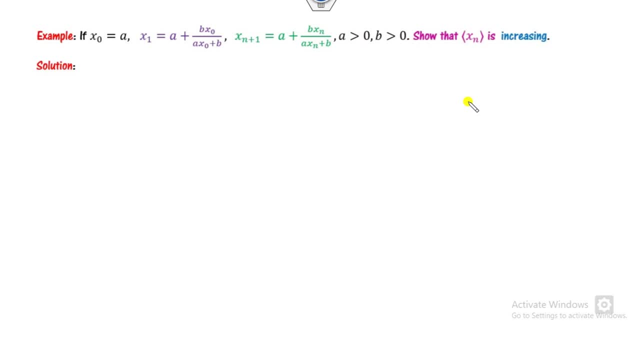 sequence is my monotonically increasing sequence, while a, i's are my monotonically decreasing sequence, are the required answers. Look what the similar nature are there. So again, x, 0 is given to a and a is my positive number. Check about the sequence is increasing. So what is given to you, x, 1, is given to you here. 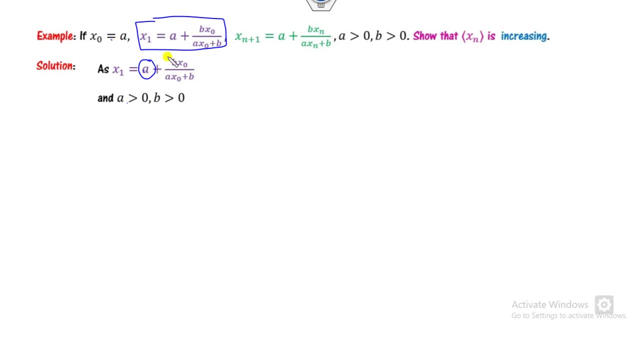 Look at that: a is my positive number, So a is positive. So x 0 is my a, So it is also the positive number. b is my positive number, So all are my positive, So that means this number is my. 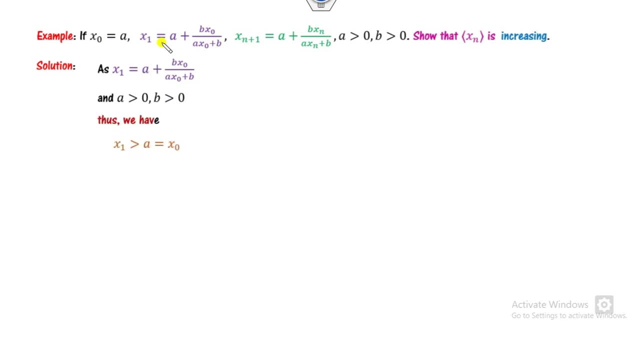 greater than 0.. Also we can say x 1 is greater than of the a. a is nothing but my x 0. That means x 1 is greater than x 0. Also we know that because all these numbers and these are my positive. So secondly, if you take 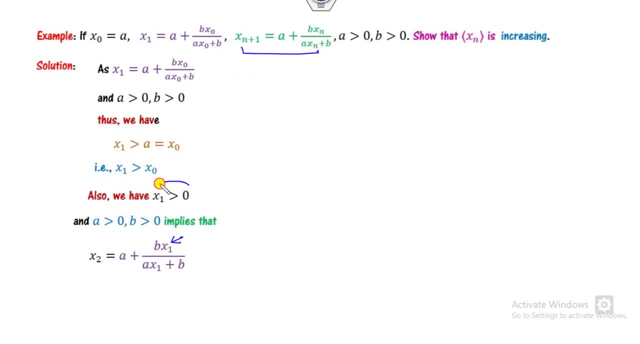 about the x 2.. So look at that: x 1 is my positive, x 1 is a, b. All are my positive. So this is my greater than of the a. So what is that? a is x 0, or you can say: this number is my greater than 0.. 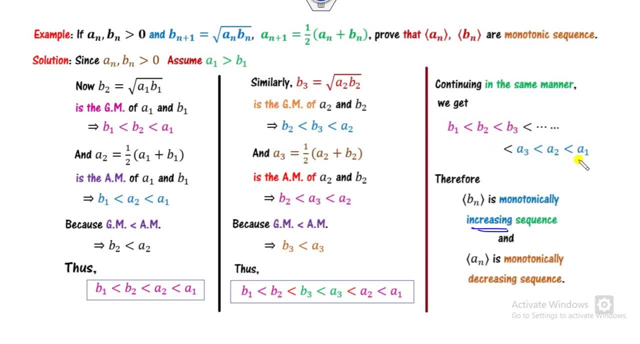 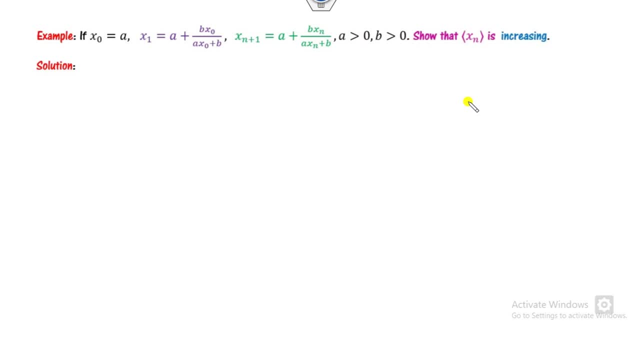 sequence is my monotonically increasing sequence, while a, i's are my monotonically decreasing sequence, are the required answers. Look what the similar nature are there. So again, x, 0 is given to a and a is my positive number. Check about the sequence is increasing. So what is given to you, x, 1, is given to you here. 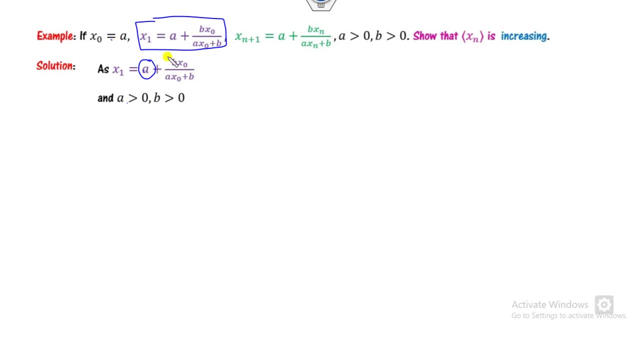 Look at that: a is my positive number, So a is positive. So x 0 is my a, So it is also the positive number. b is my positive number, So all are my positive, So that means this number is my. 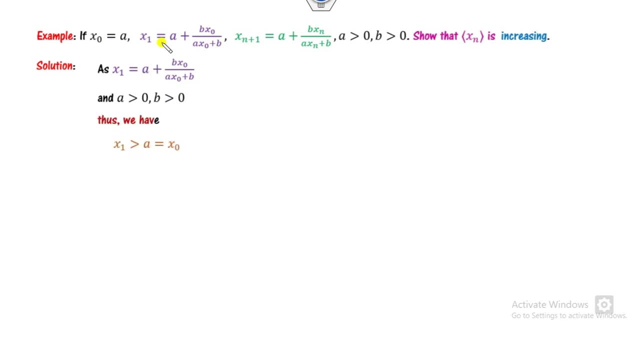 greater than 0.. Also we can say x 1 is greater than of the a. a is nothing but my x 0. That means x 1 is greater than x 0. Also we know that because all these numbers and these are my positive. So secondly, if you take 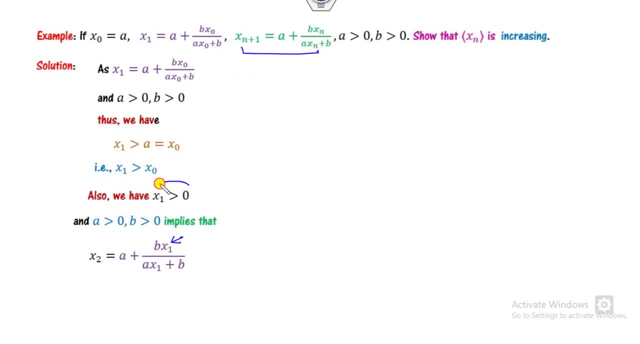 about the x 2.. So look at that: x 1 is my positive, x 1 is a, b. All are my positive. So this is my greater than of the a. So what is that? a is x 0, or you can say: this number is my greater than 0.. 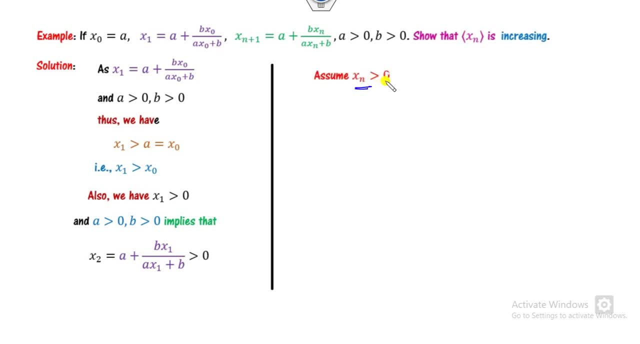 Now, once you know that, assume x n is also the positive. So what you could, what you say: x n is positive, a n is positive, So a, this is my positive. Now, in order to check whether it's increasing or decreasing, we can start from here. So if you take the LCM, you will get here When. 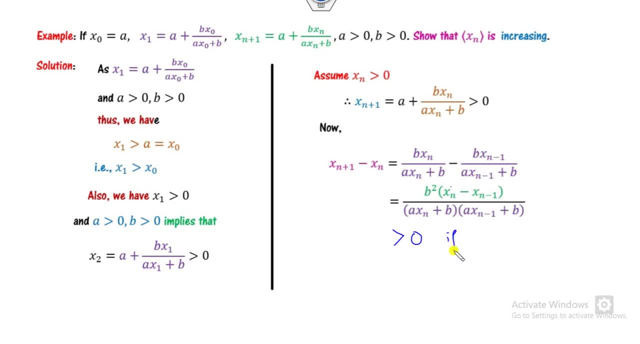 it will be greater than 0?. It will be greater than 0 only when x n is greater than of the x n minus 1.. So that means this sequence is monotonically increasing only when this condition satisfies. Look about this. 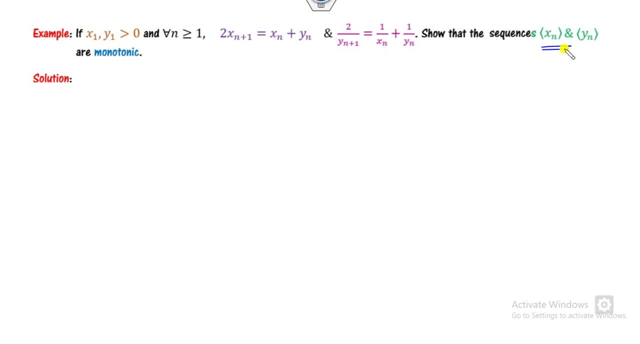 Another one here again of this kind. you have to target of this: x 1 is greater than 0.. y 1 is greater than 0, given. But what is the relation between them? Either this or this. It is not given to you. So I assume that x 1 is greater than y 1.. So once here, you can substitute this: 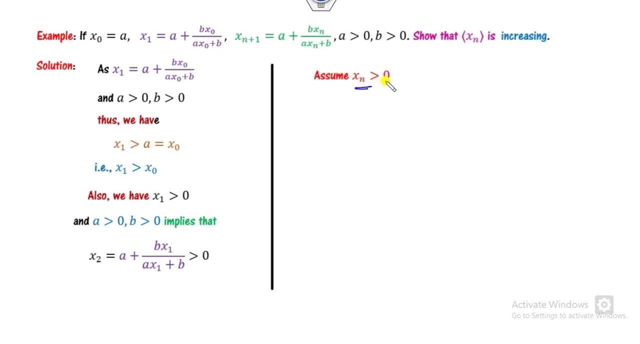 Now, once you know that, assume x n is also the positive. So what you could, what you say: x n is positive, a n is positive, So a, this is my positive. Now, in order to check whether it's increasing or decreasing, we can start from here. So if you take the LCM, you will get here When. 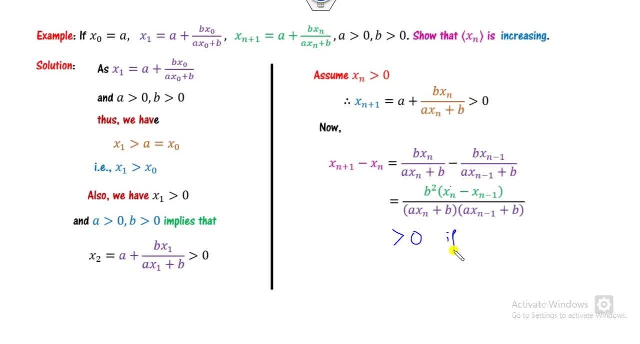 it will be greater than 0?. It will be greater than 0 only when x n is greater than of the x n minus 1.. So that means this sequence is monotonically increasing only when this condition satisfies. Look about it. 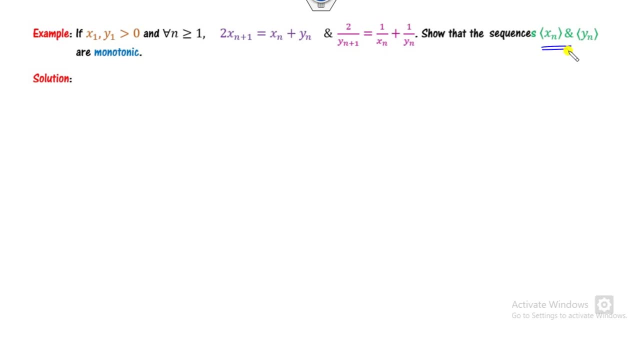 Look about it. Another one here again of this kind you have to target of this: x 1 is greater than 0.. y 1 is greater than 0, given. But what is the relation between them? Either this or this, It is not. 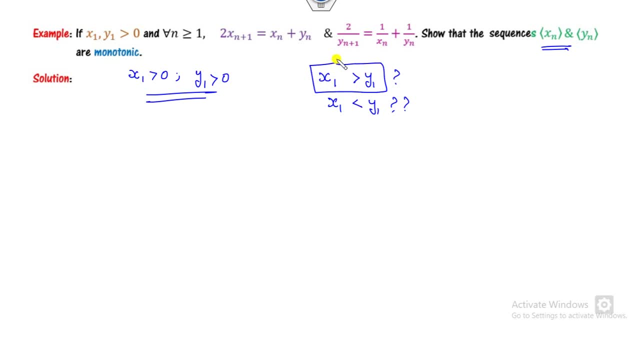 given to you. So I assume that x 1 is greater than y 1.. So once here you can substitute this value. Firstly, I can take n is y 1.. So what is that? This is 2 x 2, is x 1 plus y 1.. So 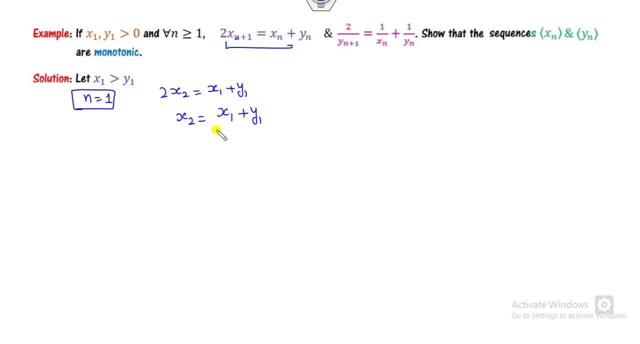 what is x 2? x 1 plus y 1 upon 2.. What is the meaning of that? What is the meaning of this? This is: x 2 is the arithmetic mean and y 2 is the harmonic mean, And since x 1 is greater than of, 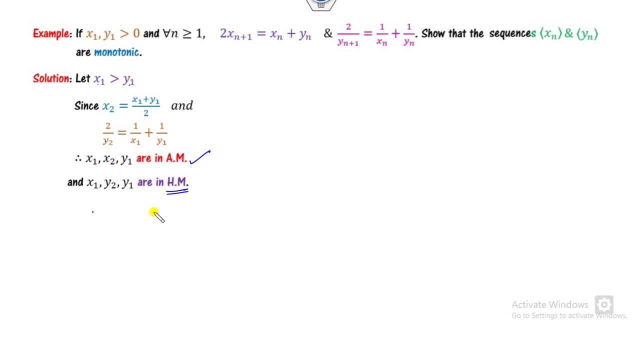 the y 1,. I can write like this: So what is the meaning of that x 1 is greater than of the y 1 and arithmetic mean always lies in between them. So we can write like this way, Similarly for: 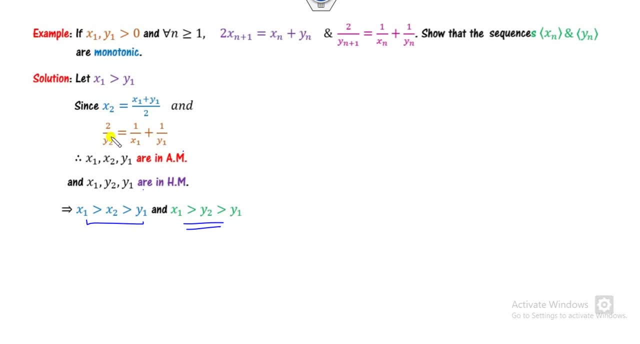 here. What is the relation between them? Either this or this, So we can write like this way. So what is the relation between the y 2 and x 2? We all know arithmetic mean always greater than of the harmonic mean. So here, So can you combine these three? You can see x 1 greater. 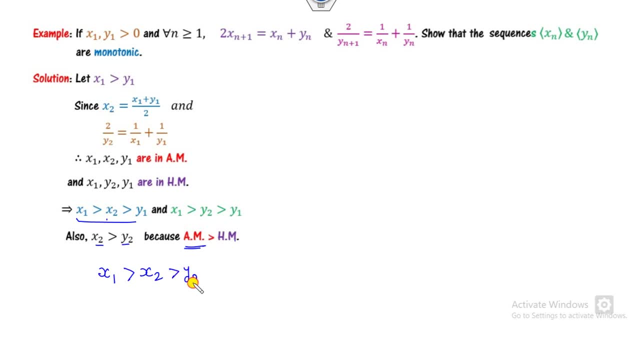 than x 2. from here, x 2 greater than y 2.. y 2 greater than y 1.. Similarly, if I take n is my 2. for the second case we can substitute here We will get x 3 and the y 3 as the arithmetic mean. 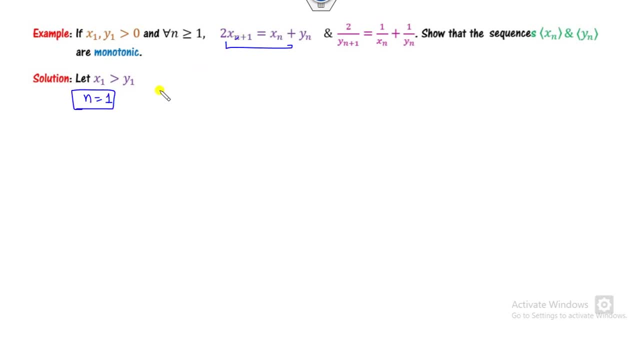 value. Firstly, I can take n is y 1. So what is that? This is 2 x 2 is x 1 plus y 1. So this is x 1.. What is x 2? x 1 plus y 1 upon 2.. What is the meaning of that? What is the meaning of this? 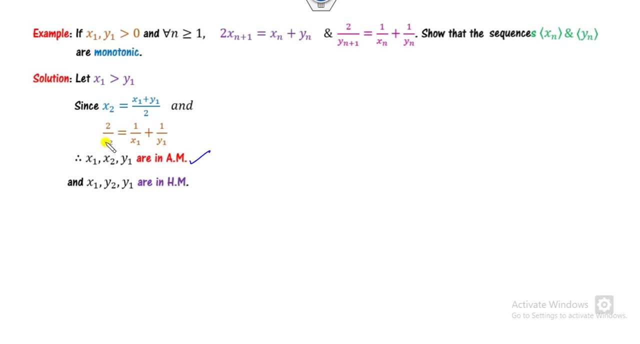 This is: x 2 is the arithmetic mean and y 2 is the harmonic mean. And since x 1 is greater than of the y 1, I can write like this: So what is the meaning of that x 1 is greater than of the y 1? 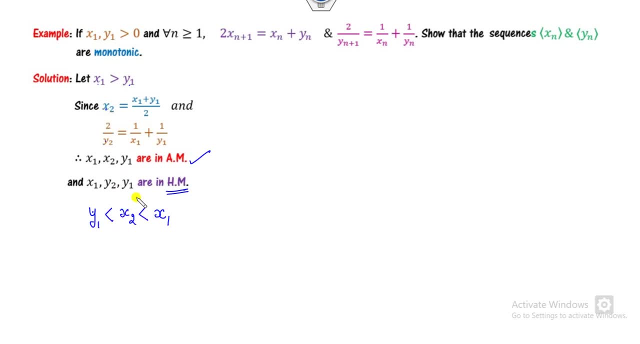 and arithmetic mean always lies in between them. So we can write like this way: Similarly for here: What is the relation between the y2 and x2? we all know arithmetic mean always greater than of the harmonic mean. so here: so can you combine these three? you can see x1 greater than x2. from here, x2 greater than y2. 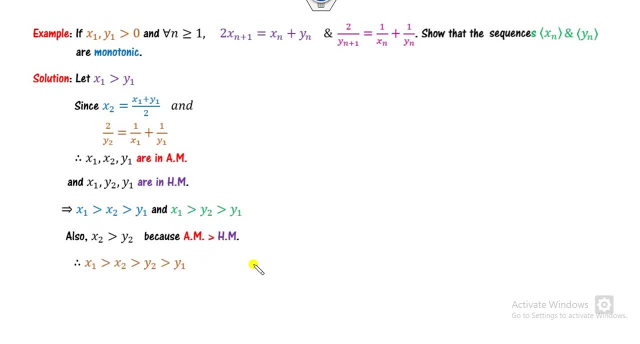 y2 greater than y1. similarly, if i take n is my 2. for the second case we can substitute. here we will get x3 and the y3 as the arithmetic mean, geometric mean. as we see, x2 is greater than y2, x3 is the harmonic mean, arithmetic mean, and is my here. so from this again we can deduce that 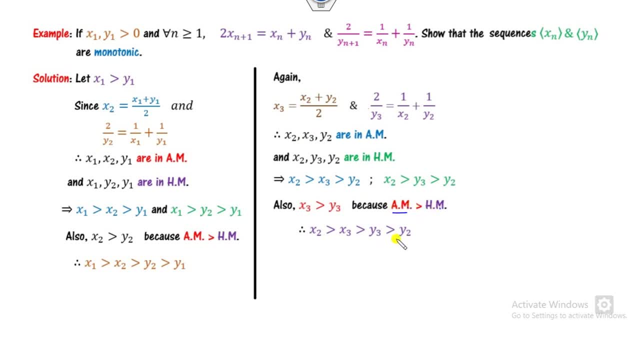 as harmonic mean is less than of the arithmetic mean. we can get here so clearly: sees: x1 is greater than x2, x2 greater than x3. we can combine them here. we can see this similarly for the y component and in the similar manner we can. 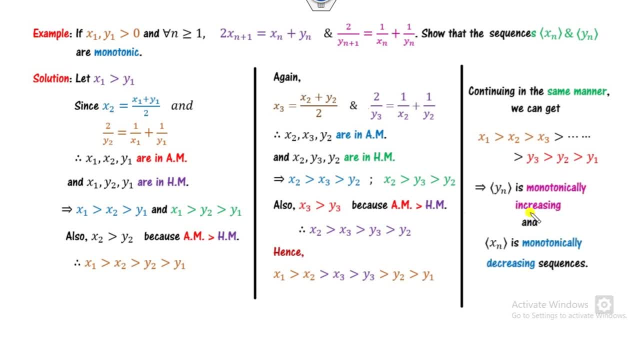 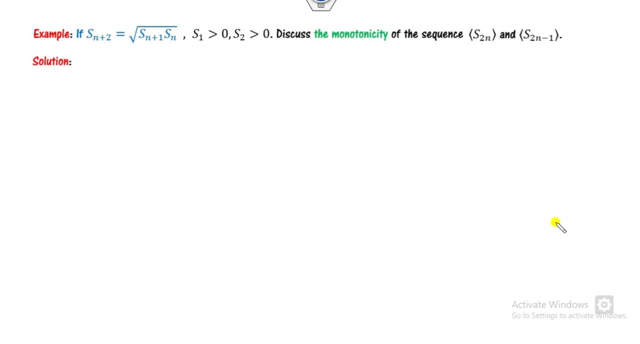 get, as this sequence clearly says that x i is my decreasing sequence and y i are my increasing sequence. are there? look about the another one. so again you have to check the monotonicity of sequence. so clearly says that if you take s1 and s2, both are positive. but again, either. 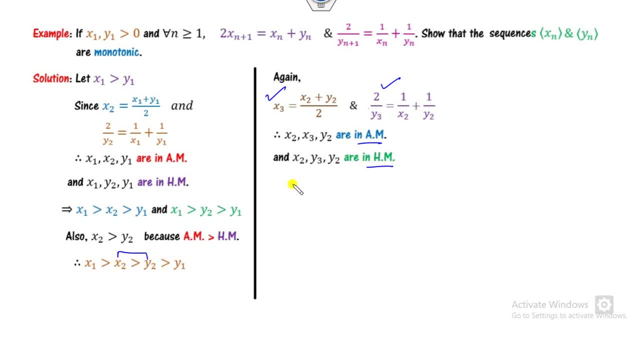 and geometric mean. As we see, x 2 is greater than y 2.. x 3 is the harmonic mean, arithmetic mean and is my here. So from this again we can deduce that, as harmonic mean is less than of the arithmetic, 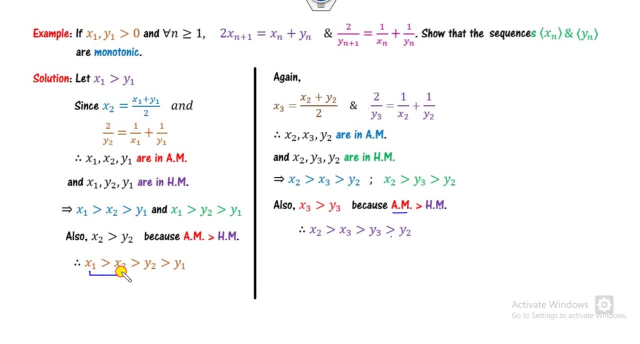 mean we can get here So clearly see, is x 1 is greater than x 2.. x 2 greater than x 3, we can combine them here. We can see this Similarly for the y component And in the similar manner we can get, as this sequence Clearly says, that x i is my decreasing. 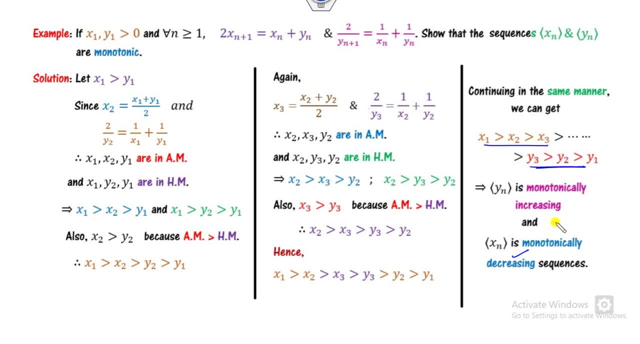 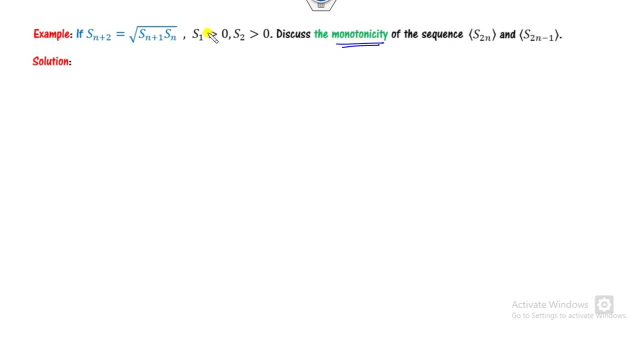 sequence and y i are my increasing sequence. Look about the another one. So again you have to check the monotonicity of the sequence. So clearly says that if you take s 1 and s 2, both are positive. but again, either this happen or this happen. You can take any one of them. So 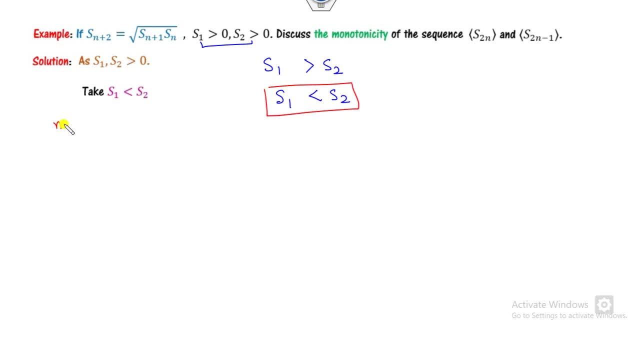 let us say in this time, I consider So let us say that x 1 is greater than x 2.. x 2 greater than x 3, this one. So if I take n is my 1, in here you get s 3. are this? What is the meaning of that? 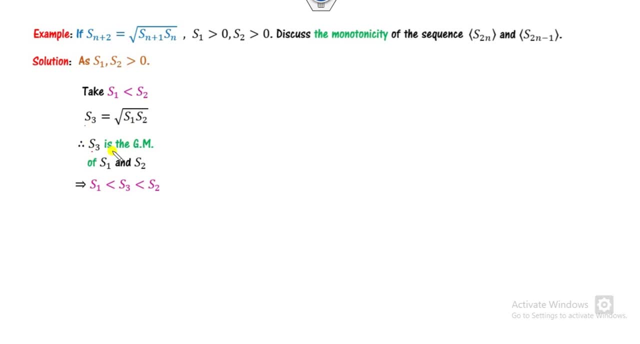 This is nothing but my geometric mean. So once s 3 is my geometric mean and s 1 is less than of the s 2, I can write here Similarly. if I consider another one, s 3 is less than of this. So for n is: 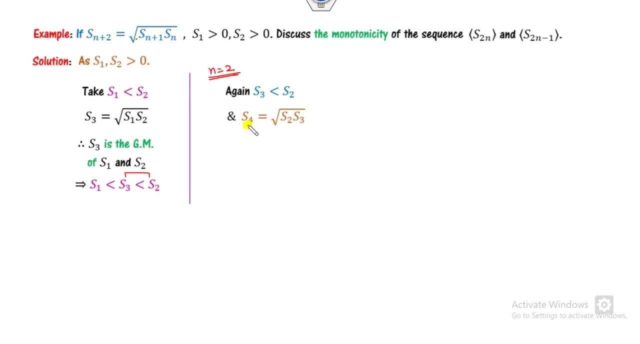 equal to 2, I can substitute here this. So what is the meaning of that? This is my geometric mean: s 3.. So s 3 is less than of s 2,. I can write s 4 in between them, So can you write the combined. 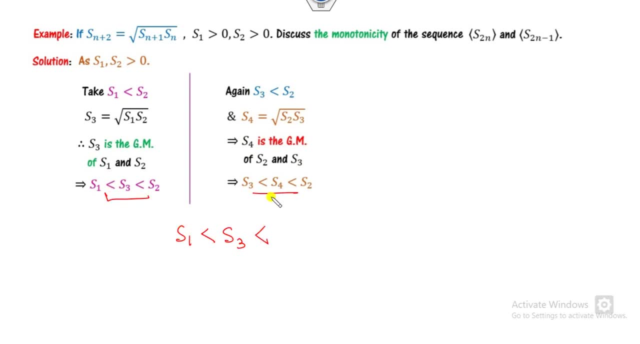 of this. Yes, you can do s 3.. s 3 is less than of the s. 4 is less than of s 2.. Similarly, you can extend them. You can see, this is the 1,, this is a 3, then 5 and so on, and it is here. So it means. 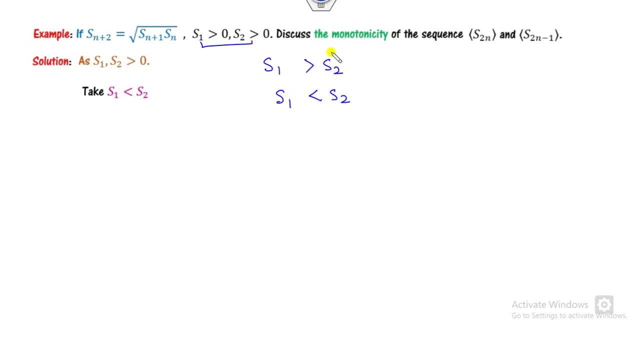 this happen or this happen, you can take any one of them. so let's say, in this time i consider this one. so if i take n is my 1 in here you get s3, are this? what is the meaning of that? this is nothing but my geometric mean. so once s3 is my geometric mean and s1 is less than of the s2, i can write. 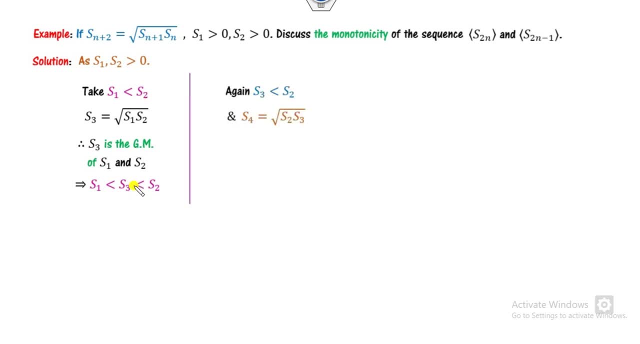 here. similarly, if i consider another one, s3 is less than of this. so for n is equal to 2. i can substitute here this. so what is the meaning of that? this is my geometric mean of s2 and s3. so s3 is less than of s2, i can. 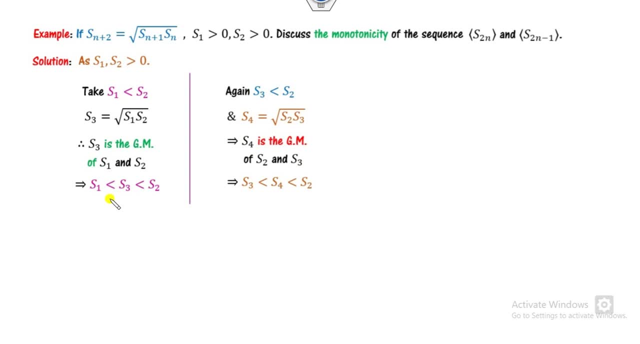 write s4 in between them. so can you write the combine of this? yes, you can do s3. s3 is less than of the, s4 is less than of s2. similarly, you can extend them. you can see this: the 1 is a 3 then. 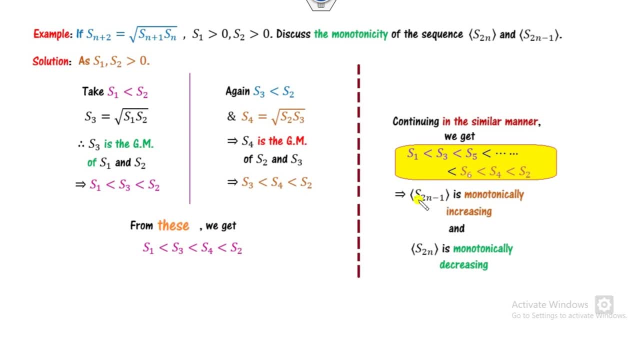 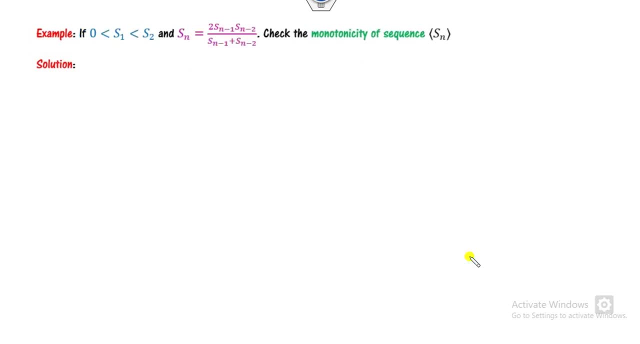 5 and so on. and it is here. so it means the odd sequence is my increasing, while the even sequence is my decreasing. look what the another one are there. so in this case it is given that s1 is my positive, s2 is greater than s1, which is positive again. so look at that. it is already mentioned that. 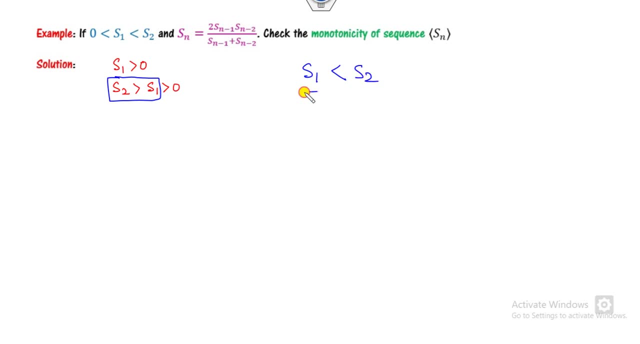 it is already mentioned that s1 is less than s2. so we can firstly reformulate that i can rewrite this form as of this- what is the meaning of that? so i can write this form as of this and i can write to this: so again, s3 is less than of the s2. so from here we can do this again: call the one and then we can see that if i also want to leave some one. and then we think that s2 isder keiner apart from ours, and this will be �1, which means I'll take 2 and divide by 2, which means that I can do t1, I will take n, and due to opportunity, and here we can do, i will take t2という relatedholism, and that means falling over the part of t2. but there it is also. 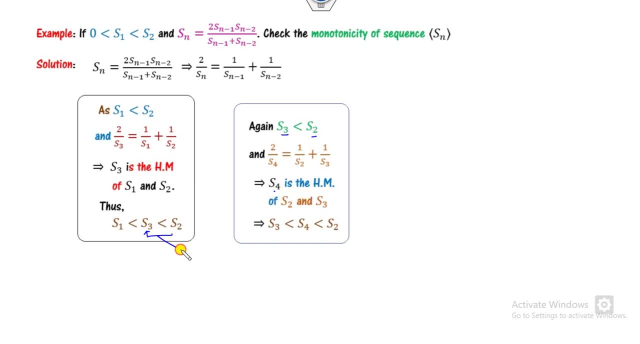 got as S4 as a harmonic mean and so on. Can you combine them? You can easily combine them. S1 is less than S3, less than S4, less than S2.. Similarly, we can generalize them and we can get as the: 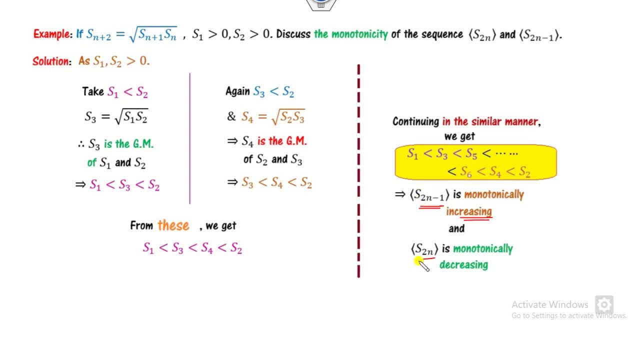 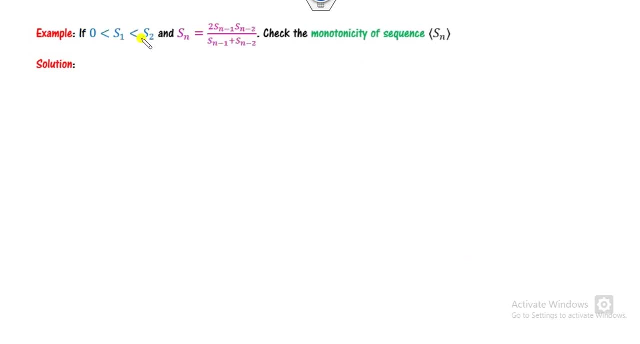 the odd sequence is my increasing, while the even sequence is my decreasing. Look what the another one are there. So in this case it is given that s 1 is my positive, s 2 is greater than s 1, which is positive again. So look at that. It is already mentioned that.